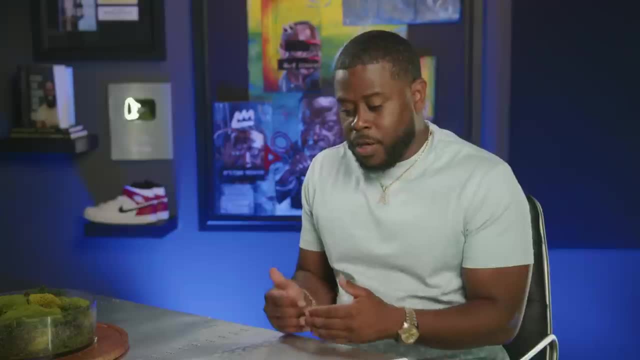 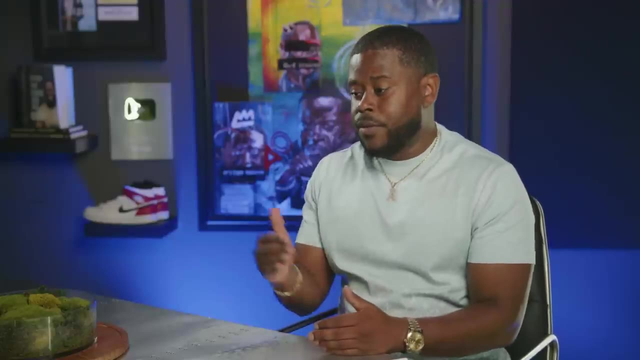 attached to it. I have an assignment attached to it. Hey, I'm giving you this. This is what I need back in return. When I give it to a friend, hey, I'm giving it this. This is what I need back in. 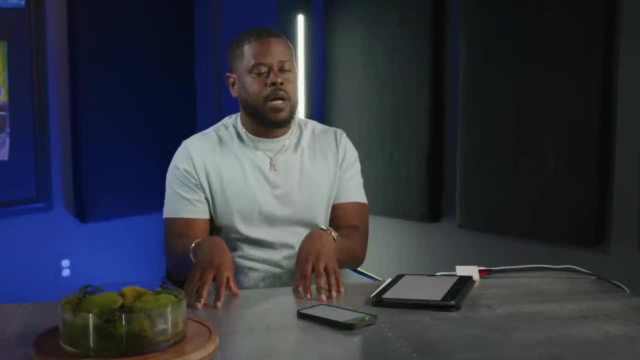 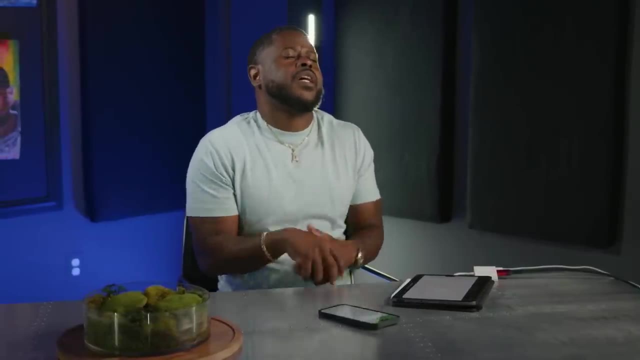 return. I know where every dollar of my money is going. And a part of me is going to say this, And I know some of y'all are going to cringe And I know some of y'all are going to be like what in? 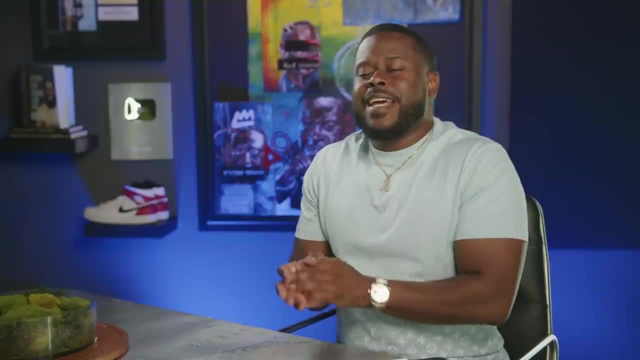 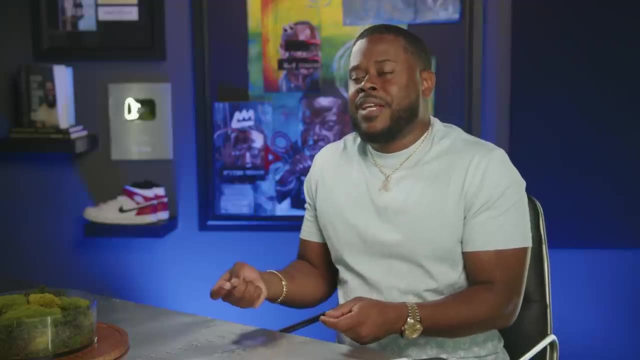 the world, Anthony. But not budgeting is not a sin. Let me say that again: To us Christians, not budgeting is not a sin. To us Christians, not budgeting is not a sin. To us Christians, not budgeting is not a sin, but it is bad stewardship. How do you expect God to give you a quarter? 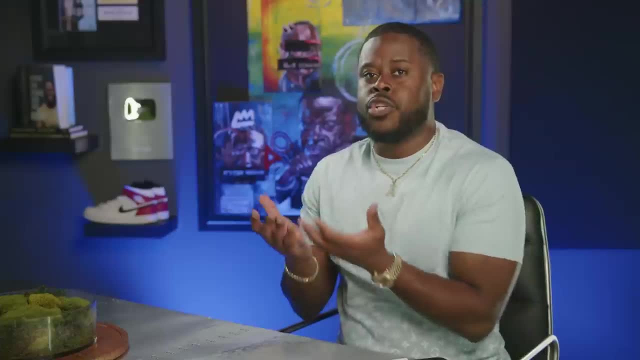 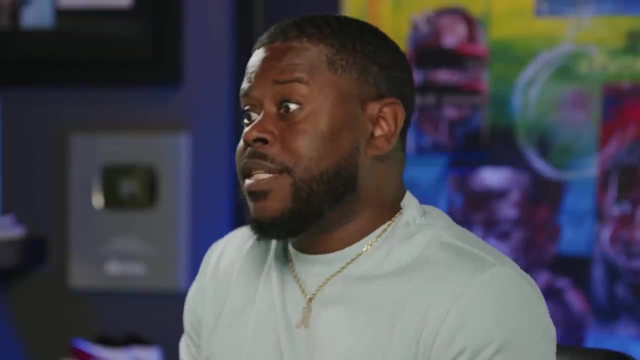 million dollars a year And you don't even know how to control the quarter million dollars a year. but you're asking God to give you more money, but you're not even taking the time to sit down and actually budget. You're not even taking the time to sit down and say: you know what God? 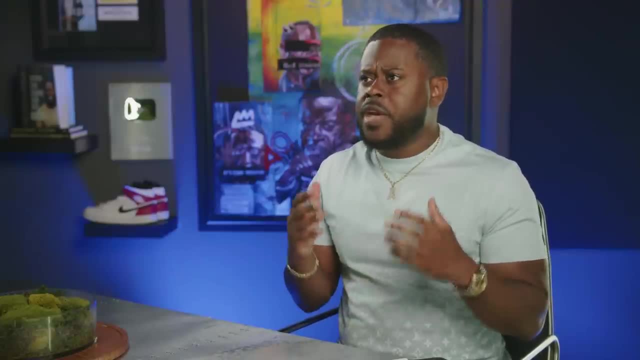 I know you gave me this, this $50,000 a year. God. I know you gave me this, this $80,000 a year. God. I know you gave me this $650,000 a year. God. I know you gave me this $650,000 a year, God. 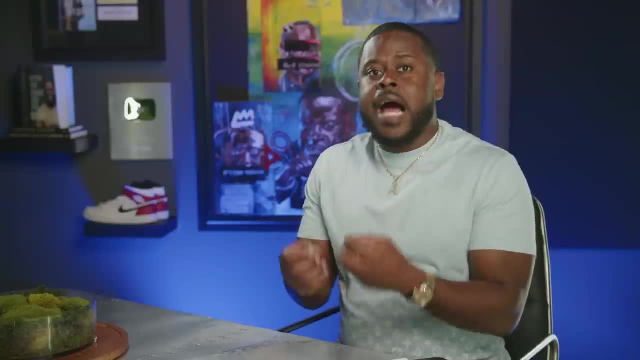 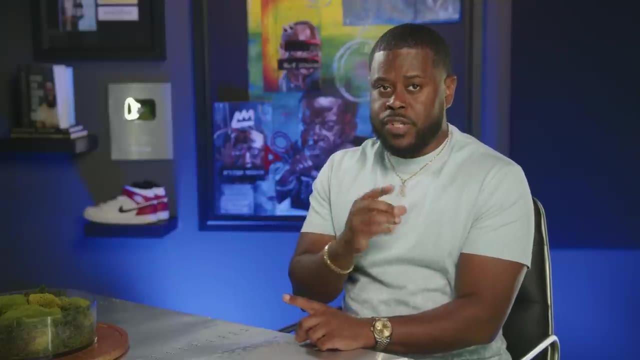 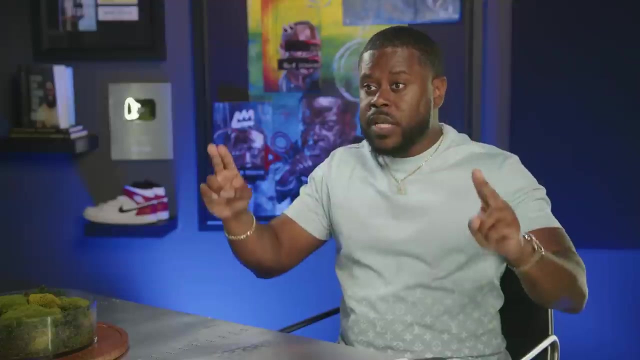 this six figure a year, God, and I'm going to show you that I am going to steward this money well, because here is the truth, you guys, the Bible says: Christians, if we're practicing a Christian faith, the Bible says: give 10% back. Cool, Great. Then a lot of us get twisted. 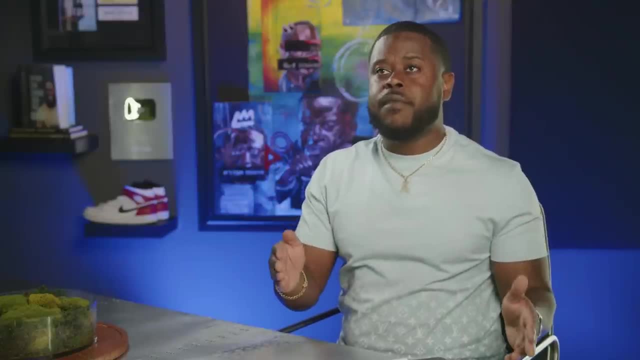 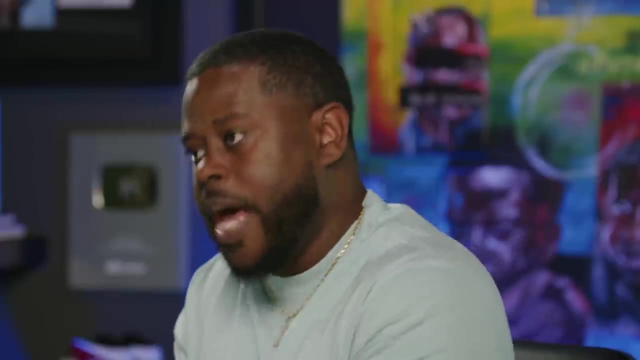 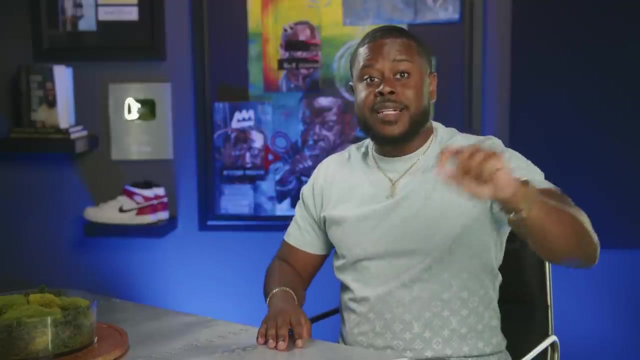 We're given a 10, but we're thinking the other 90% of it is ours. No, we're just called to manage that well, And you cannot manage 90% well if you're not taking the time to sit down and put it on paper. The Bible says it clearly: where there is no vision, 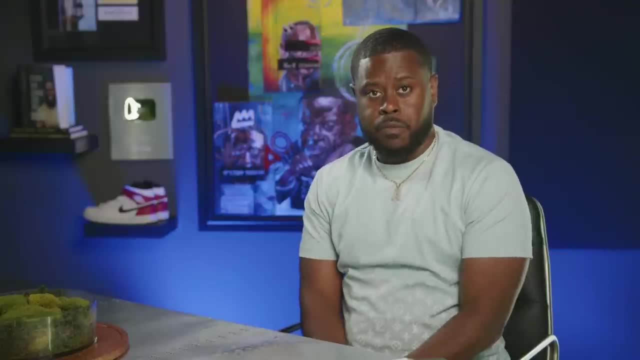 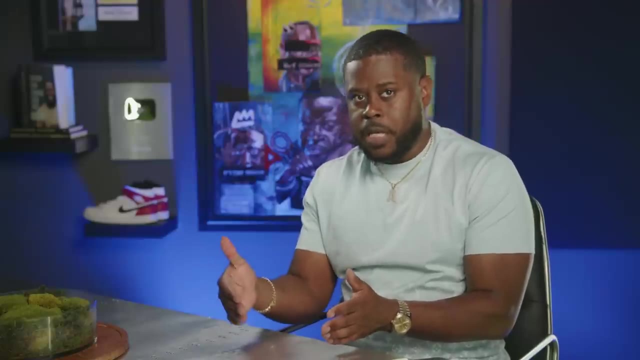 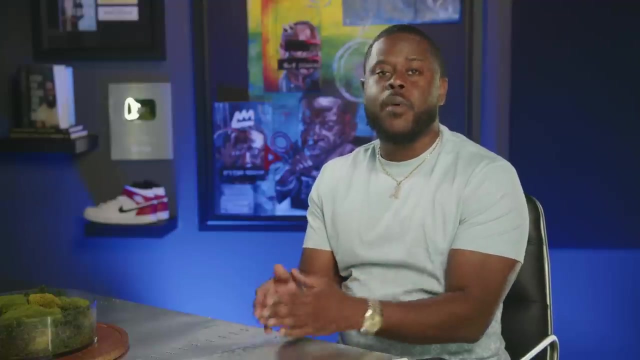 written down. that's where people perish. So where there is no vision for your money, where there is no plan for your money, where there is no system for your money. that's why you're broke. And so today, I literally want to break down how I budget, how Anthony O'Neill budgets his money. 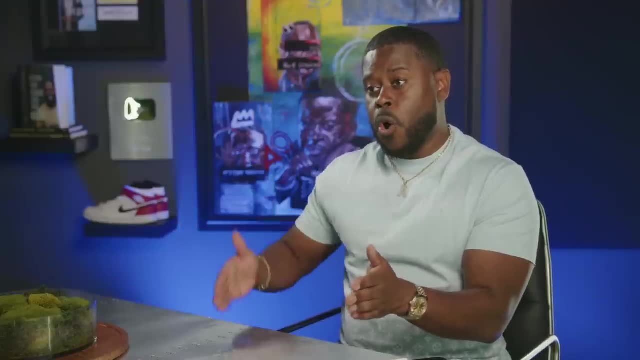 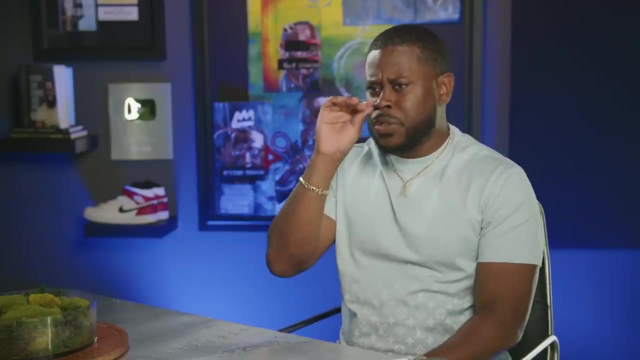 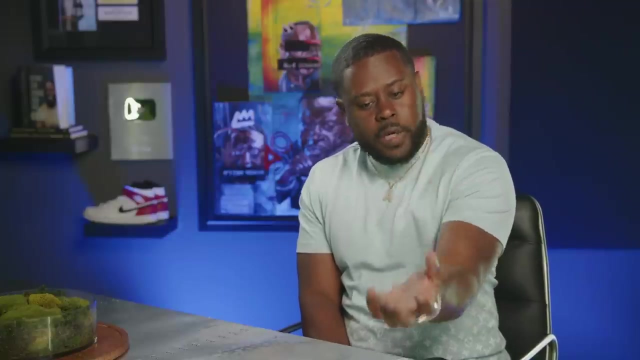 how I spend every dollar on paper, just so that I can have freedom to enjoy my money. A budget doesn't mean that you're broke. No, a budget means that you care about the finances and the resources that God put into your hand. And so because you care about it, 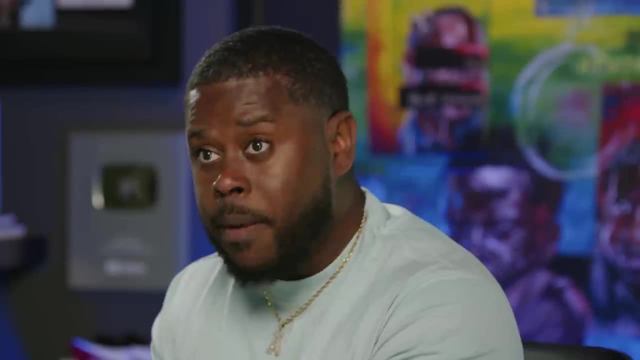 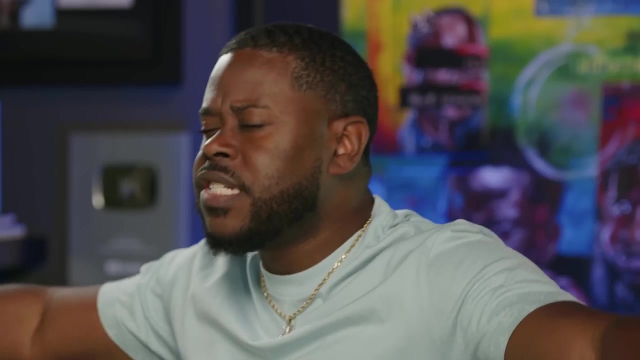 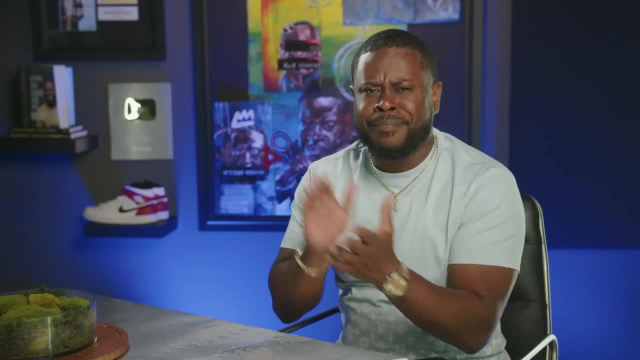 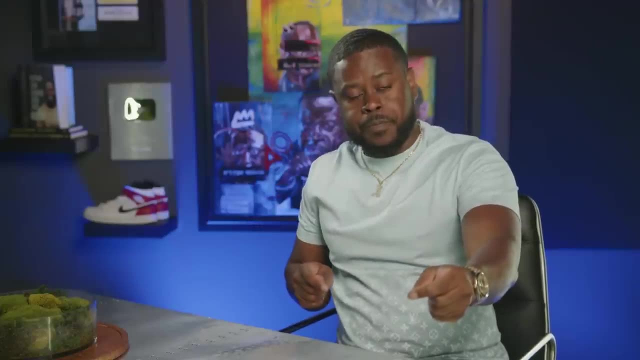 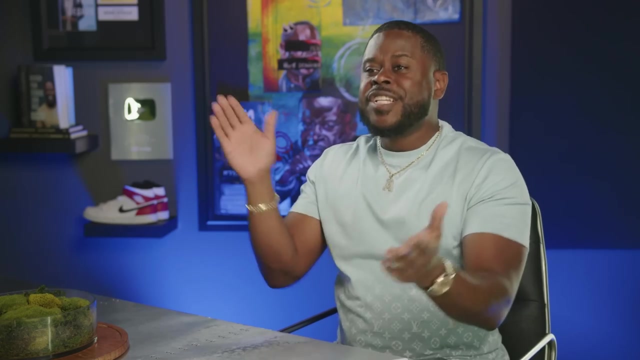 doing that at all. But isn't it funny when you walk into a bank they say, do you have? what A business plan before they give you their money? And God is simply saying the same thing Like yo, if you want me to give you more, give me and show me. you know how to operate off of a plan. 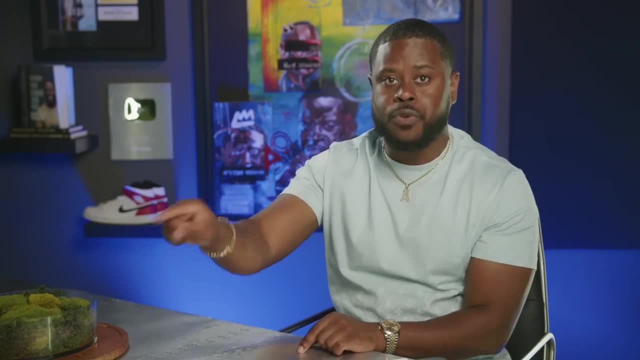 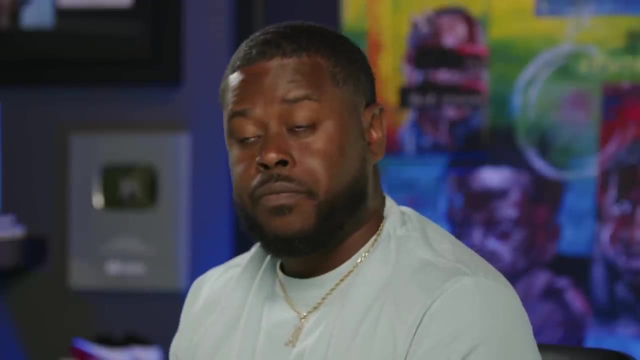 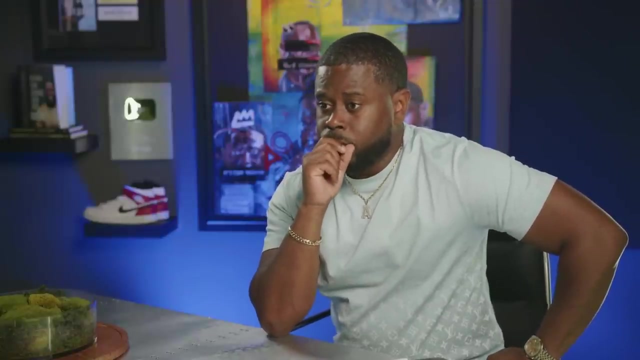 before I give you money- Not before I loan you money- before I give you some of the resources that I have, I want to make sure that you can steward it Well. some of y'all are a budget away from a pay raise. I'm speaking spiritually. 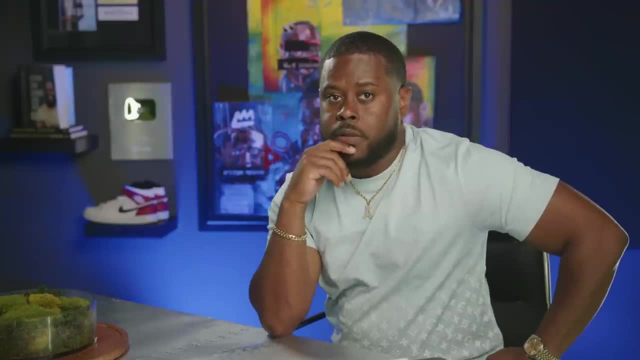 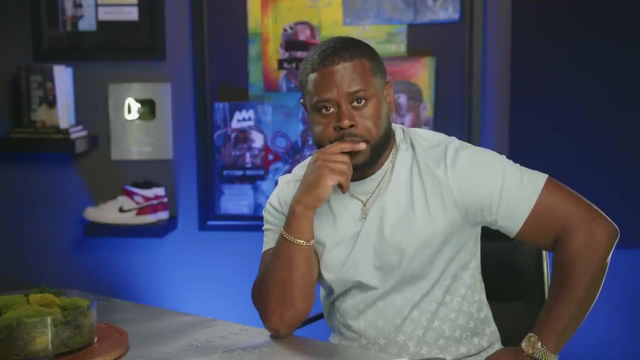 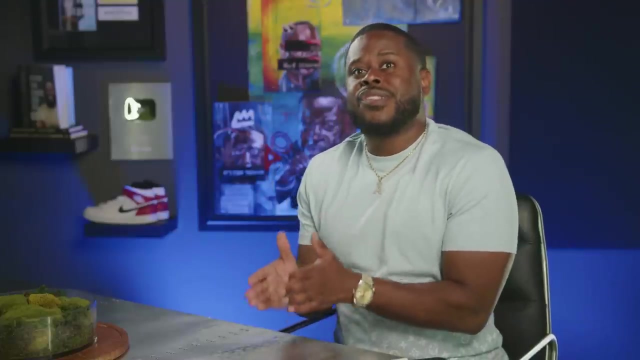 Some of us are a budget away from making a million dollars. Some of us are a budget away from getting that business off the ground. Some of us are a budget away from my first home. God is waiting for us just to see if we can just simply budget and put a vision on paper. 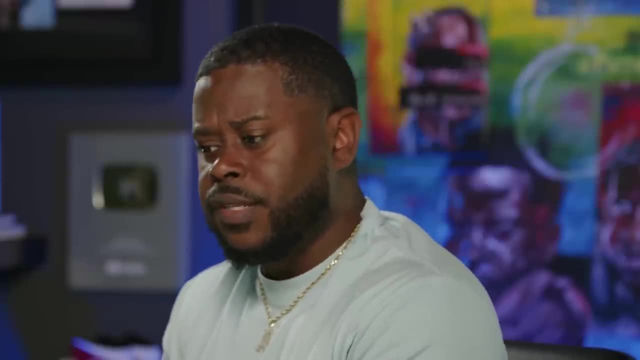 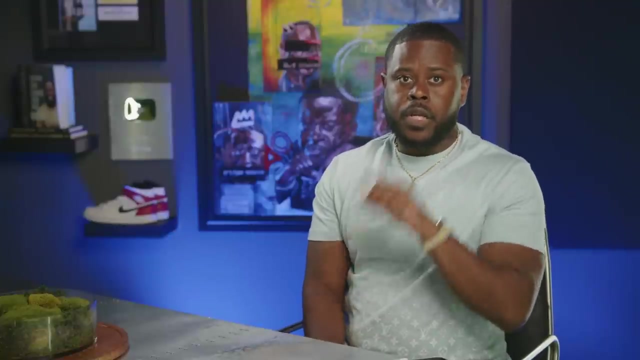 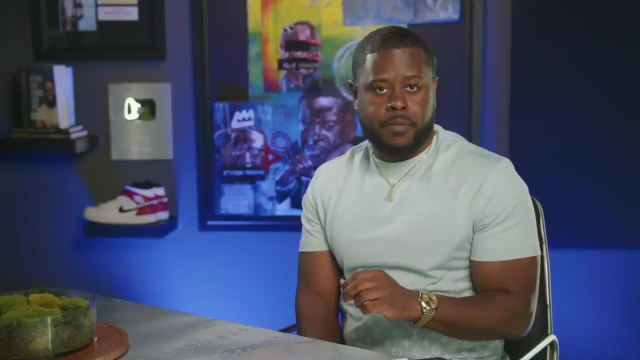 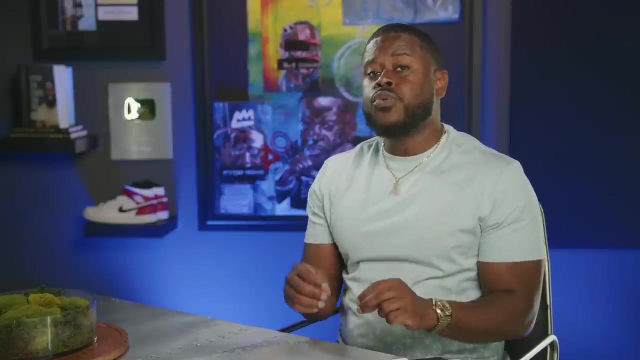 to make sure that if he gives us that pay raise, that if he gives us more income, we're going to be all right. So today I'm going to show you how to simply base- not base. how to simply budget your money. just basic basic. just basic math on what to do using the, the, every dollar. 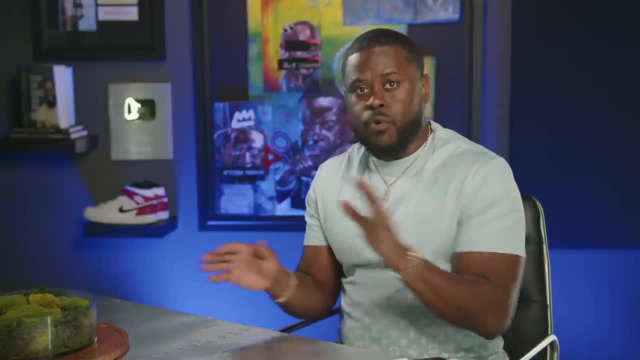 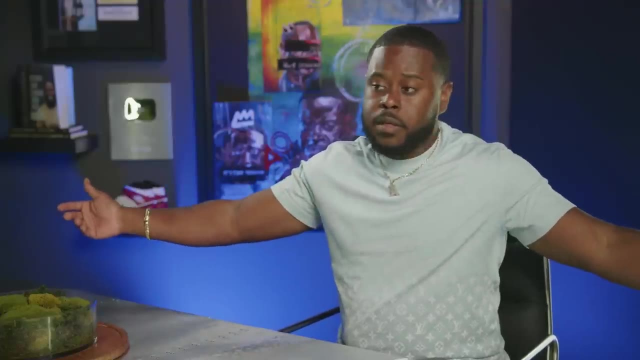 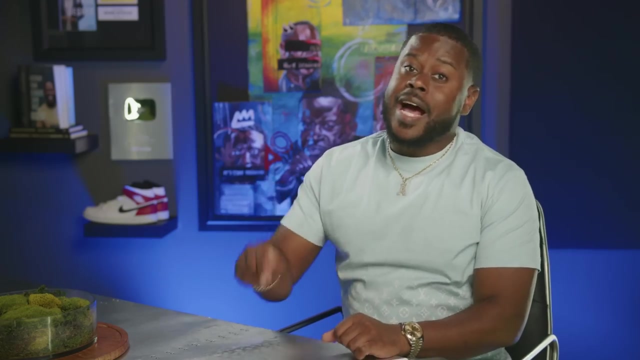 zero base budget formula. I said every dollar because I use the app called every dollar. I still use it. I still rock my boys and my family and and my sisters over there at Ramsey solutions Cause I think that their every dollar app is the best app because literally you cannot. 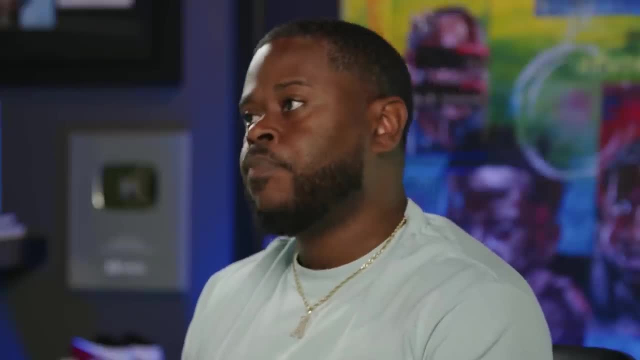 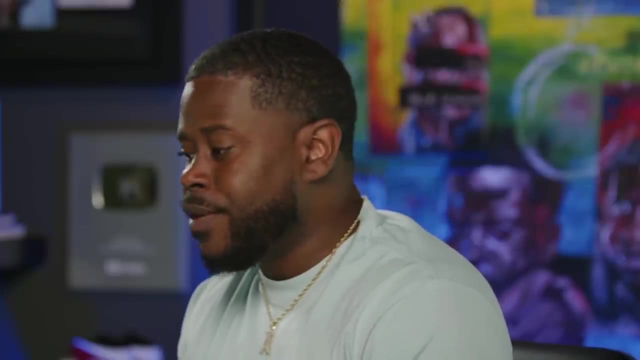 close out the app. You can't close out the app. You can't close out the app. You can't close out the app. but you cannot complete your budget until you spend every dollar on paper And this is called a zero base budget format that I use. that I highly recommend that you use. I'm going 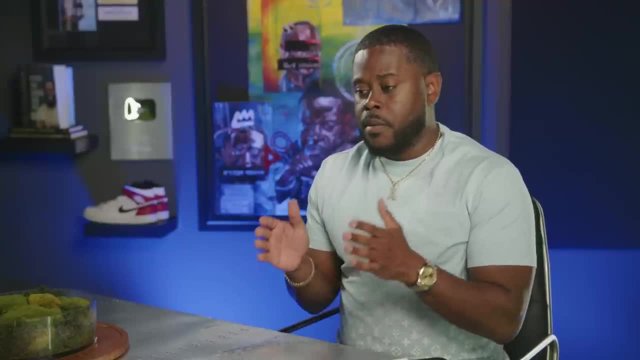 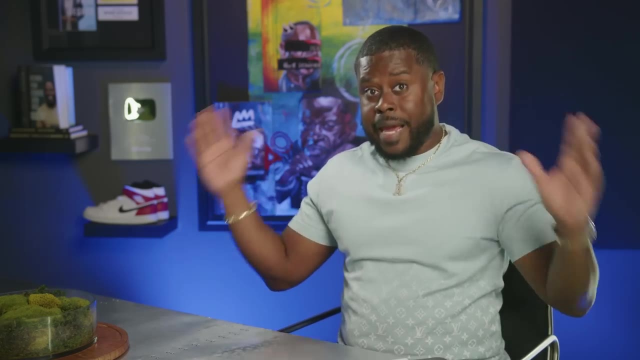 to put the link to the every dollar app in today's show notes. I want you to check it out, go download it, go rock with them. It's an amazing app. If you don't use every dollar, that's totally fine. You need to get an app to budget. If you got to do an Excel, do whatever you got to do. 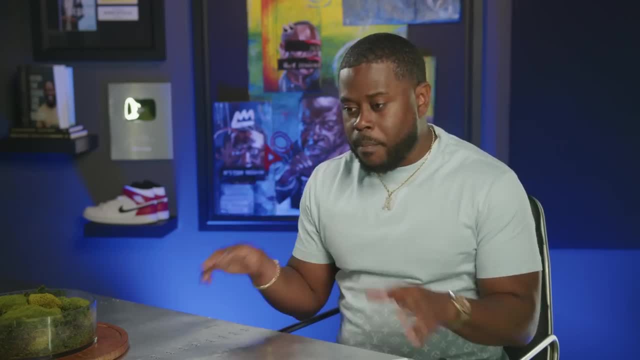 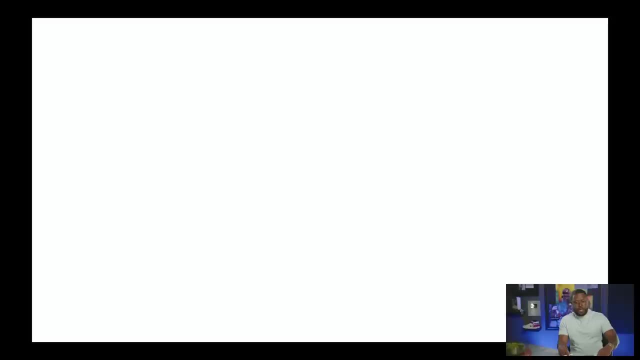 So you can do a zero base budgeting format. I promise you it will save your life. but let's send me over to my iPad real quick. Walt is our new guy man. He's helping out CJ, my main producer. He's our assistant show. 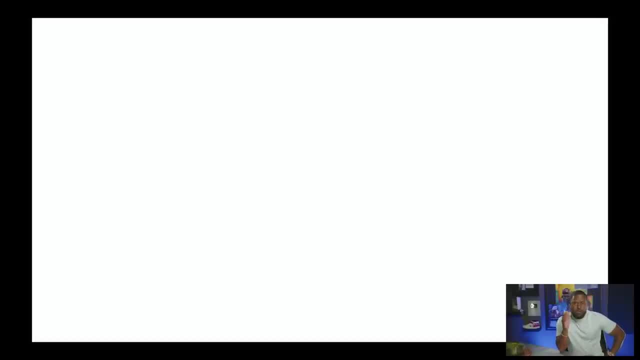 producer. video producer. and welcome Walt to the team. Drop him some love in the comments y'all. But I'm super excited because I really want to give you all the keys to to budgeting, And the very first key to budgeting is this thing: 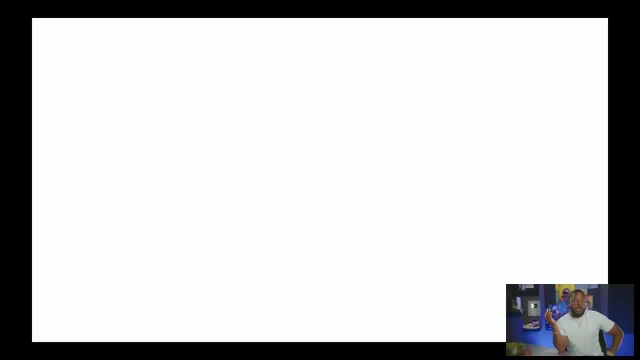 all of your income, all of your income on a sheet of paper, All right. So let's just say, for an example, let's say, just I'm going to use simple numbers, right, Simple numbers, nothing major, nothing big, but make it, make it very realistic. Let's just say: you see, I'm going to do green. 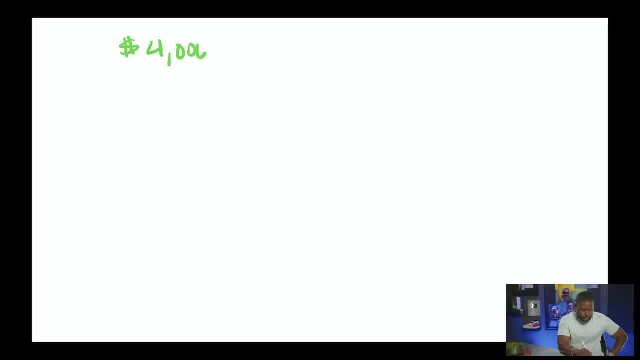 Let's just say you see $4,000 a month from your job net. All right, I'm just rounding numbers up. And let's just say you see another $1,000 a month from your side side job right Net. So let's just say you have a total of 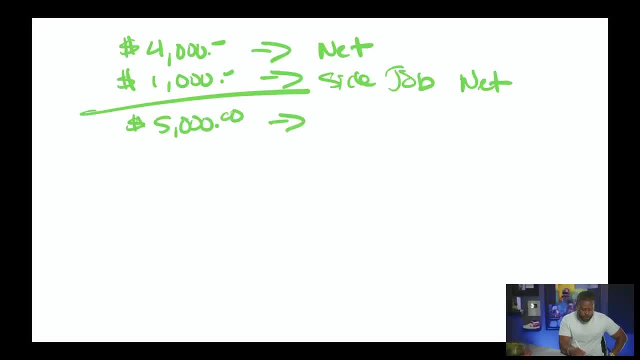 $5,000 a month in income. So the very first thing when it comes to having a zero based budget is to list all of your income, And when you list all of your income, you, you now set the stage of. this is where I'm starting. So, now that we've talked about this, is where 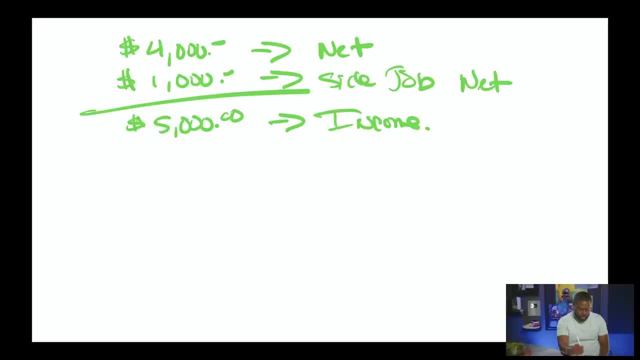 we're starting, We have an income of $5,000.. This, this is the budget that we're working with off today. All right, So the very next thing is going to be: okay, This is- I'm going to put this over here- This is our income. The very next thing is going to be: what are we giving? 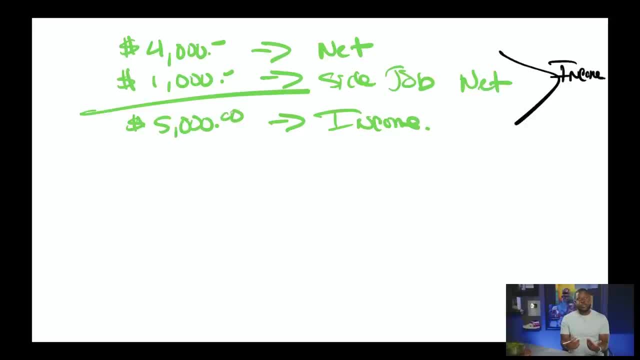 Like what, what, what are we giving? How are we being generous? You see, a lot of people get so confused: Oh man, if I give away money, I'm taking money away from myself and my family. And the truth of the fact is actually, the more you give away within your means, right, The more 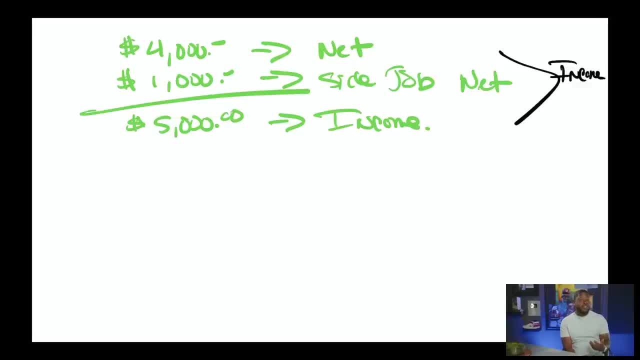 you give away, the more you're showing God how generous you are and how loving you are And, honestly, the more God wants to bless you. Wealthy people have identified one of the secrets of building more wealth is giving away as much as they possibly can within reason. So one of the 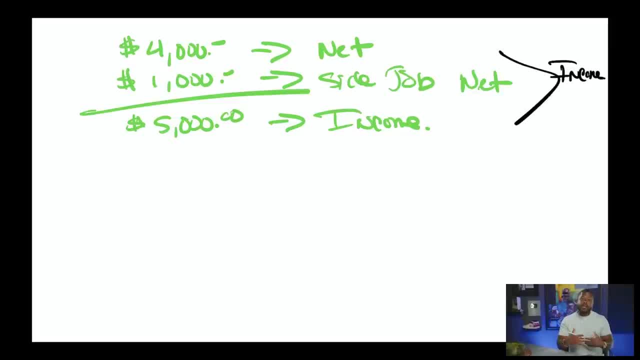 things that I do to practice. my giving is I give to my local church And I honestly give over and beyond, And so for me, if I'm at $5,000, then very next thing is I'm going to be giving away. I want you to really, really, really, really really think about it. 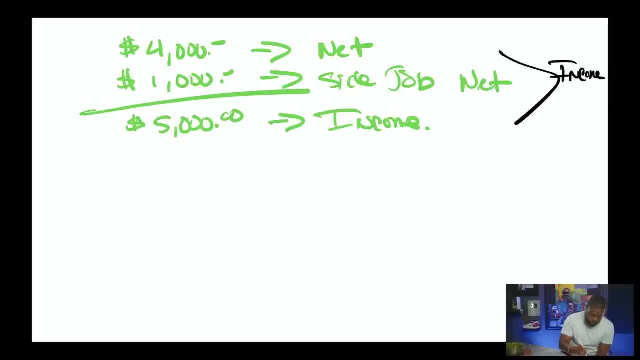 is your tithing offerings? Make sure you have the right color on here, All right. Actually, this needs to be red, because now we're going to expenses, So now we have our income, That's cashflow coming in. Expenses are cashflow going out? All right, So in red, my tithe. 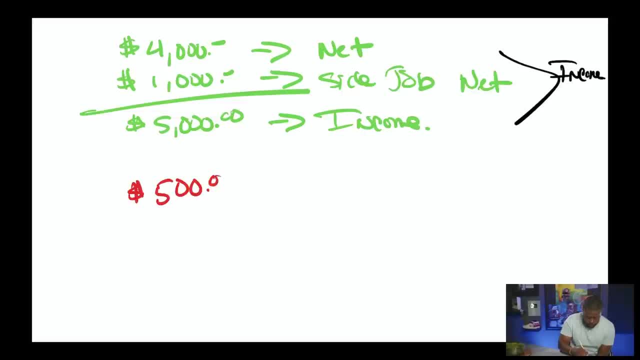 my tithe is actually going to be $500.. This is going to be my tithe, Okay, All right, So it's your tithe. So, out of the $5,000 of income that you have coming in, we're giving away $500. And 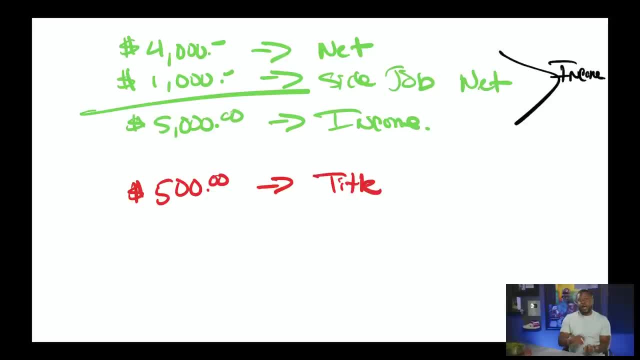 technically. I don't want to be too spiritual here, but we're giving God back $500 for kingdom building. And when we say we're giving God back $500, this is whatever church you're going to, whatever church is feeding you, whatever pastor is feeding you. 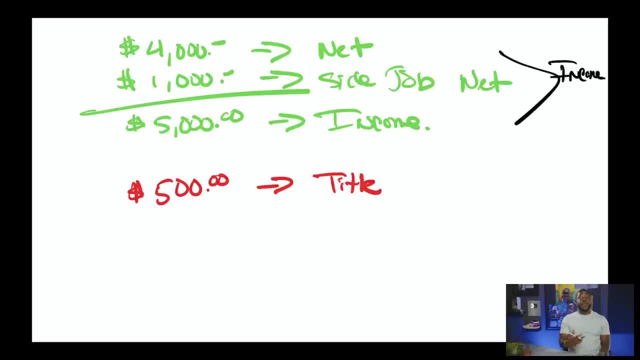 you're giving back to that local church And you're showing God that, Hey, I am being obedient to what you have set forth for us. Here is my $500 going back, And then, on top of that, you guys, I'm always going to say, give another 10% when it comes to offering, on top of your tithe. 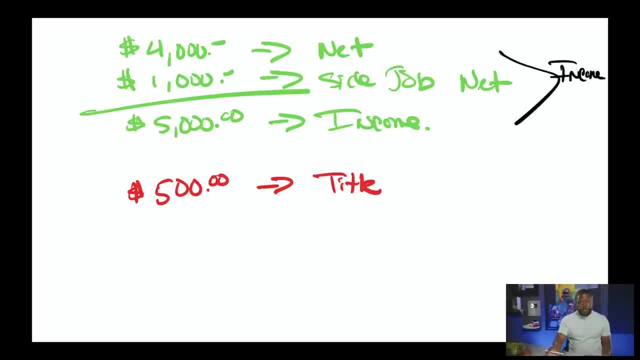 And so if you're giving $500 a month in tithe, then you're going to give- I'll say what- another $50 a month in offering. Okay, Let me make sure this is correct So y'all can understand that that's another $50. 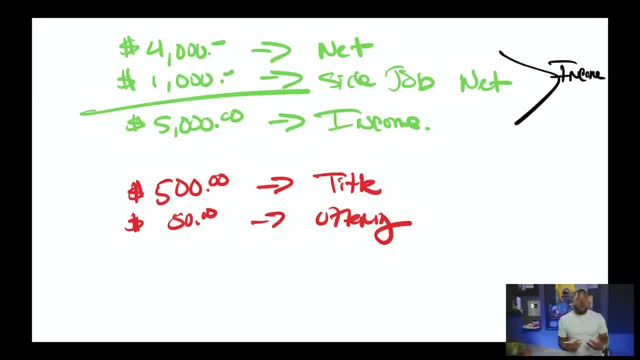 a month in offering, So that now here's what we're doing. We have income coming in, Then we have expenses going out. Our tithe and offerings are not really an expense, That is, I call that a seed, I call that being obedient, I call that being generous. 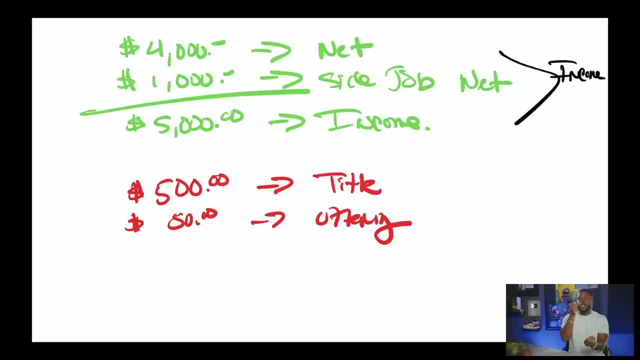 Now, what we're doing is we're activating and we're showing God that he can. he can trust us with all of our income And we're honestly saying God: not only can you trust us, but, God, you can trust me with more. The more I can give away, that means, the more you're. 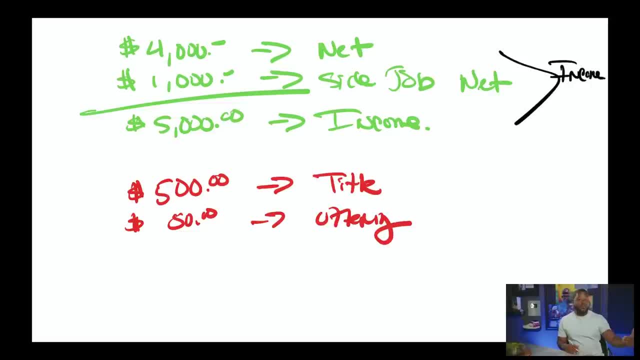 blessing me, God. So keep on blessing me And I'm a keep on being obedient. That is a secret to building wealth. We're talking about budgeting today, but this is icing on the cake. You want to build extreme wealth. You want to give more. So, after you pay God, after you're being generous, 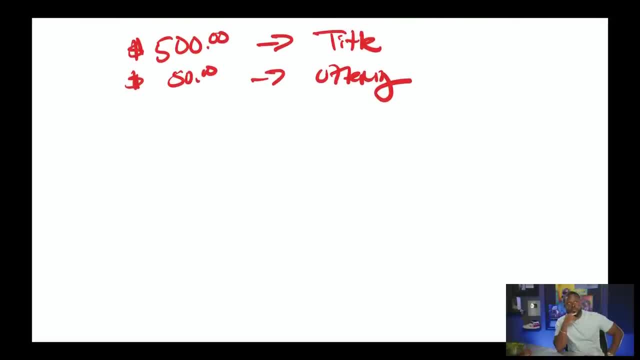 right. What's the very next thing? you, you should be paying yourself. You should be paying yourself. You should be paying into your emergency fund. You should be paying into any type of savings that you currently have. But right now I want to keep it very basic, very simple. Our goal is we should be maxing out If 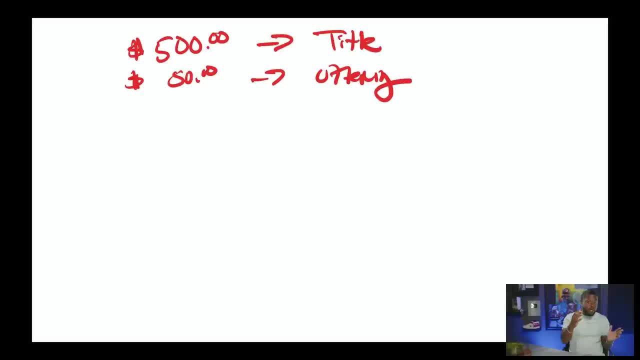 you have debt, you should be putting at least a thousand dollars to one month of expenses inside of your savings account. If you don't have debt, you should be building at least three to six months of your savings for emergencies. So I'm going to put over here. I'm going to act like we. 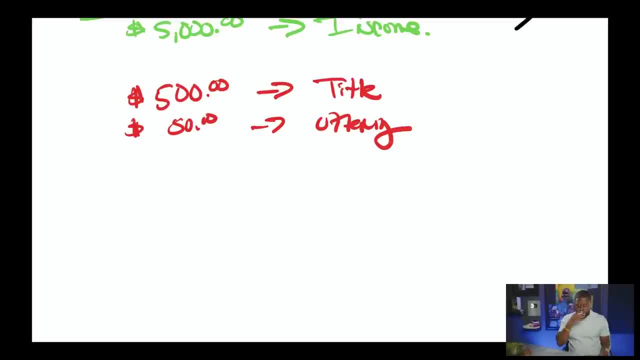 have very minimum debt, So we're not actually saving a whole lot. So I'm going to say: you know what, on a monthly basis, we are actually saving? Let's just say we're putting away $200 a month into savings because we're trying to get to the one K plus mark. right, One K plus one K. Let's say: 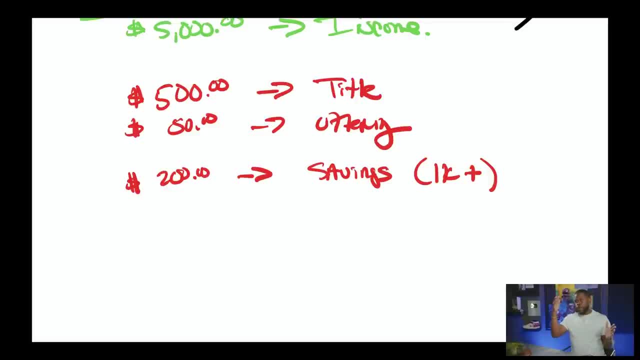 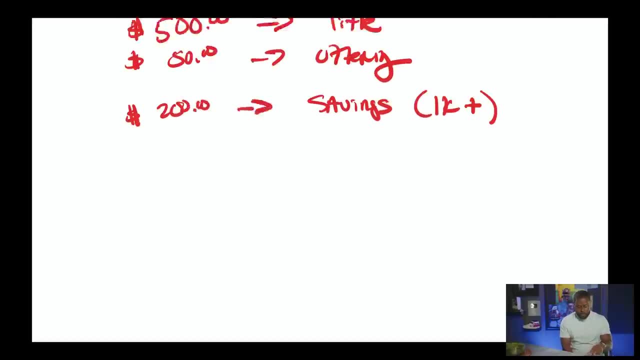 minimum to about to about one month of expenses. All right, So we are already at $750 out of the $5,000 that we have. Then from there is going to be our next thing is going to be our housing. We're going to list out everything when it comes to our housing. Now, when it comes to 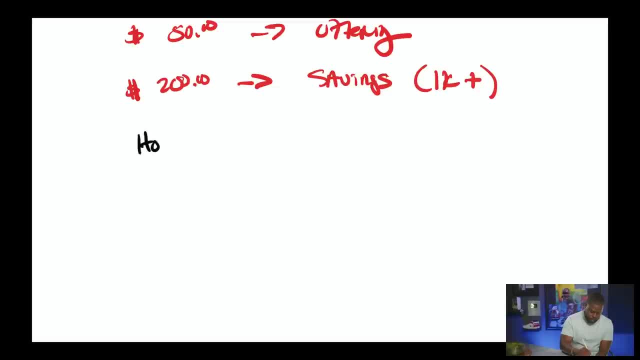 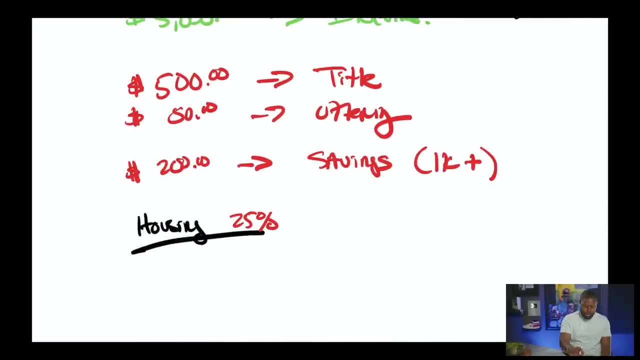 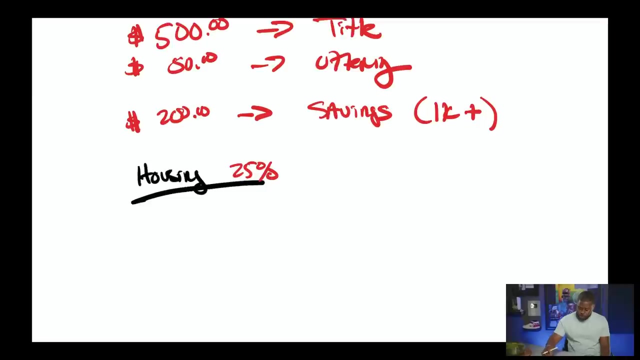 when it comes to our housing? okay, When it comes to our housing, you should be at 25% Of your take-home pay when it comes to so right here from the 5,000, you should be at 25% of your take-home pay. when it comes to your rent or your mortgage? Okay, Or your mortgage So. 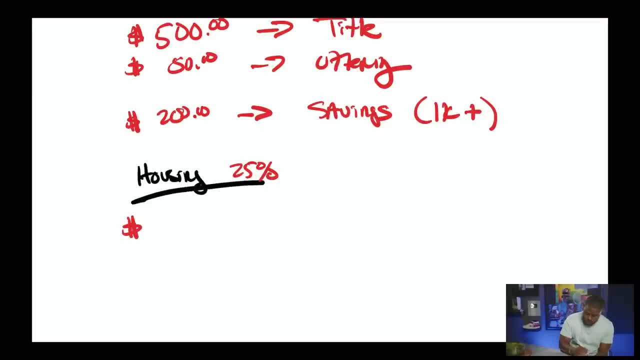 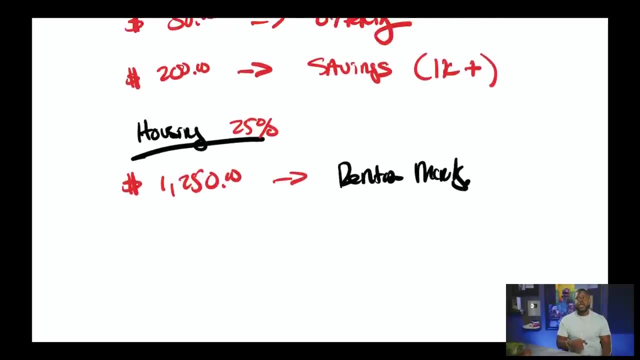 this means that your rent or mortgage should be no more than $1,250.. Okay, This is going to be rent or mortgage. Now some of y'all saying, well, is this even possible? man, I'm paying, I'm paying more, I'm paying more. 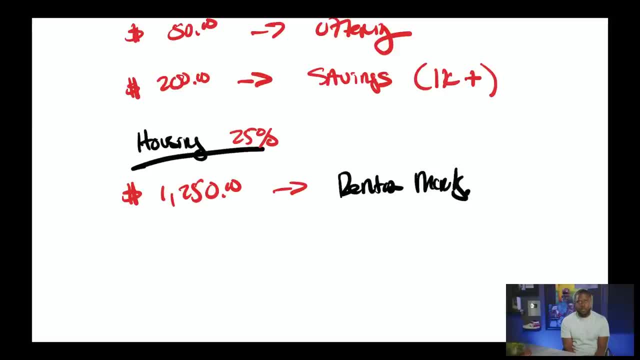 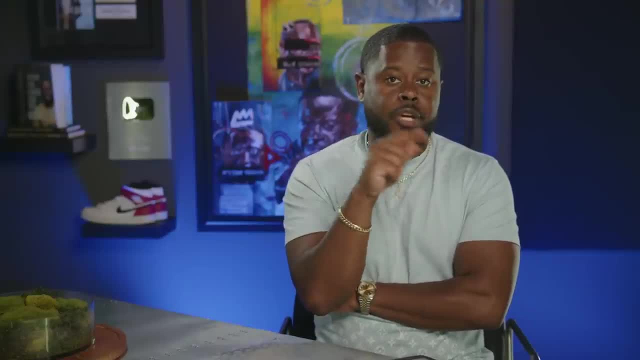 than that. Well, yes, it is possible. Here's what I am going to say, though. Can I be real with you today? I'm going to be real with you today, And those of you all listening on podcasts, I would encourage you to come over to YouTube, because I have my iPad up on the screen where I'm writing. 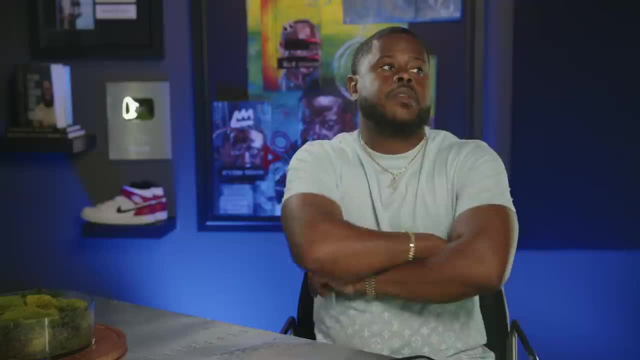 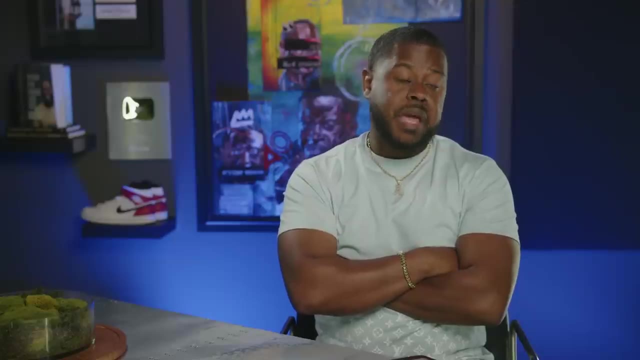 all this down, All right, And so is it possible. Yes, But is it possible that you may be living in your dream neighborhood or in your dream home? Maybe it's not. Maybe you're not living there. Is it possible that you know you may have to? miss out on your first choice of a home. Yes, Is it possible? you may have to miss out on your second choice of a home. Yes, It is possible, But here's the thing. Here's why living at 25% when it comes. 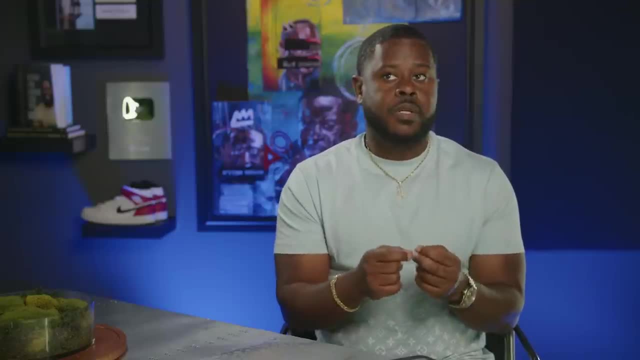 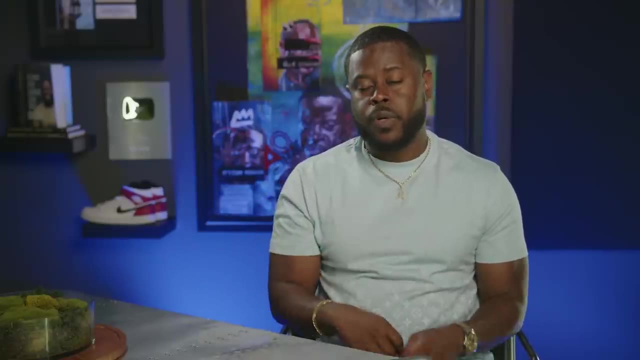 to your mortgage payment when it comes to your rent, payment is so important because you want to have margin and room to breathe, To do other things. Oftentimes, this is what I see people doing: They spend a lot of money on their homes because they want a neighborhood, because they feel like a neighborhood may not. 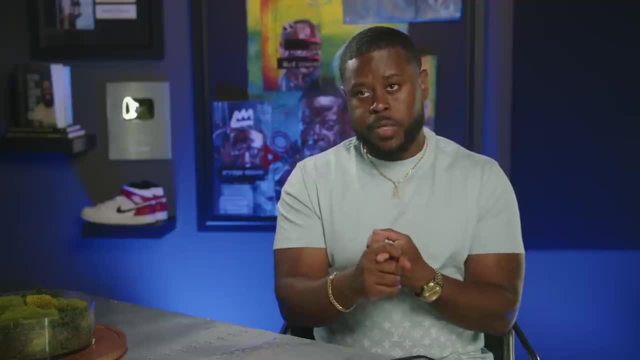 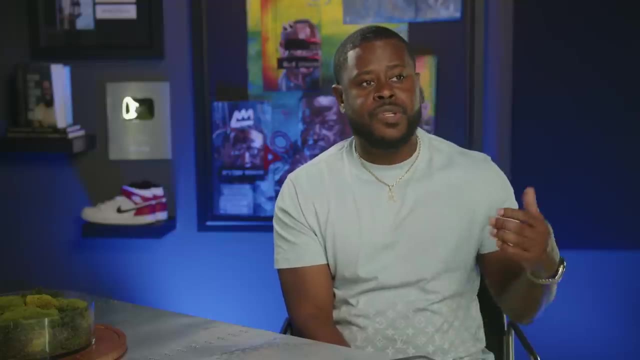 be as safe as the next, because it has some older homes in it or it may be on the older side of town. Man, that don't mean nothing. That don't mean nothing. I'm not saying move into the hood and where you're hearing shots fired every single day, But just because it doesn't have the white. 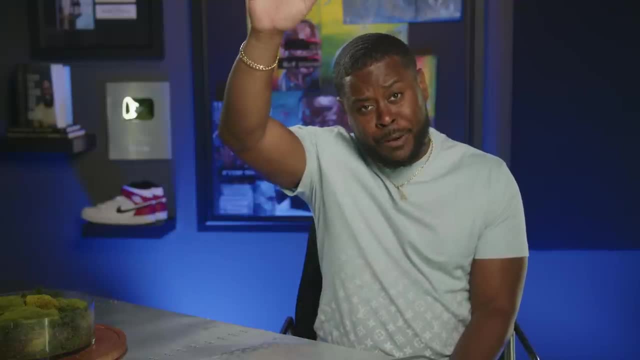 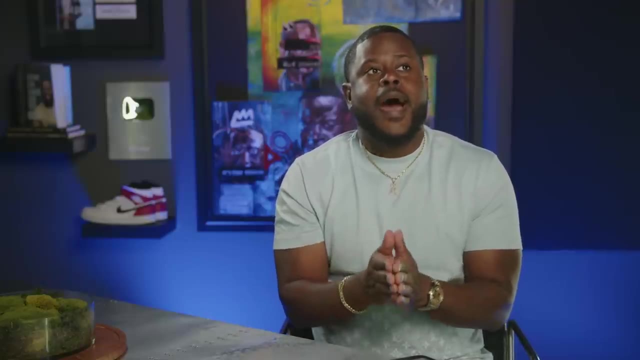 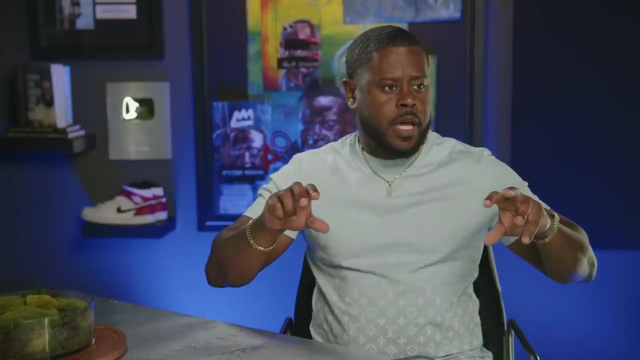 picket fence and beautiful neighbors out there saying, hey Tom, how are you? Doesn't mean that neighborhood? Some of us got to really step back and ask ourselves: how bad do we really want freedom? How bad do we really want financial options and opportunities- The greatest enemy. 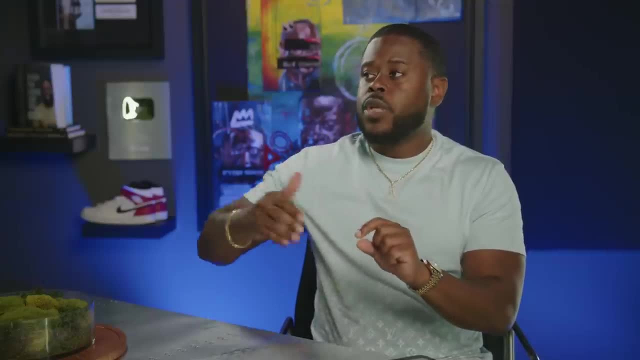 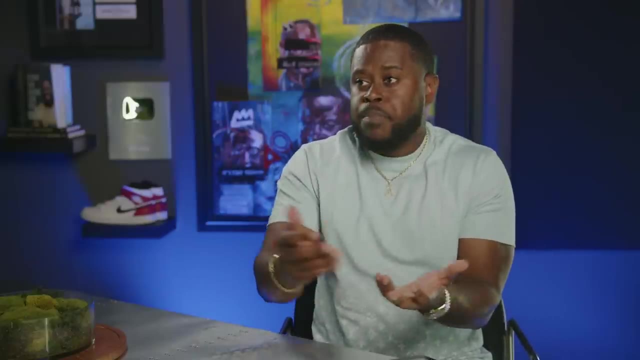 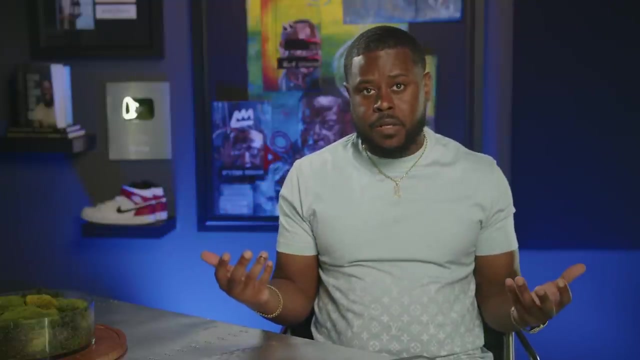 to our success. the greatest enemy to us really reaching the goals is our excuse. What's our excuse? Hey Tom, how are you? What's our excuse? The best school? What's our excuse? The best school? What's our excuse? The 100% perfect environment. Man, I live in a great neighborhood. 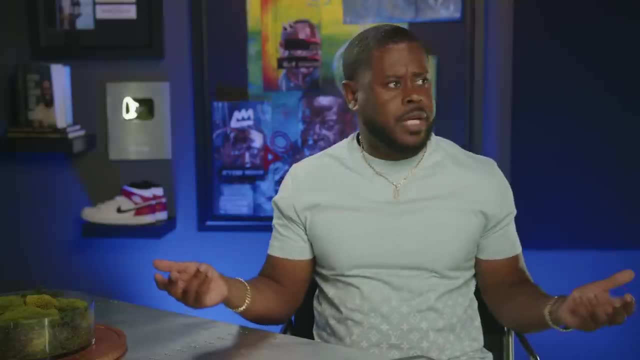 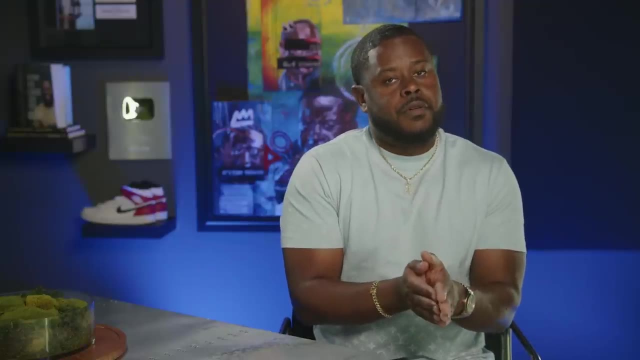 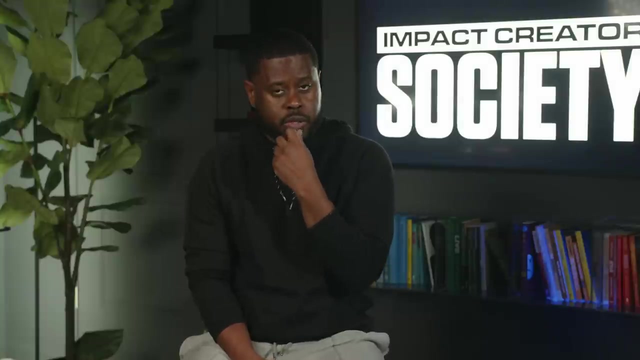 right now. Homes are still getting broken into, Cars are still getting broken into. Nowhere is 100% safe. Now let me say this again because I do understand. Studies are showing nearly right now- currently in the year 2023, that nearly 70% of people live. 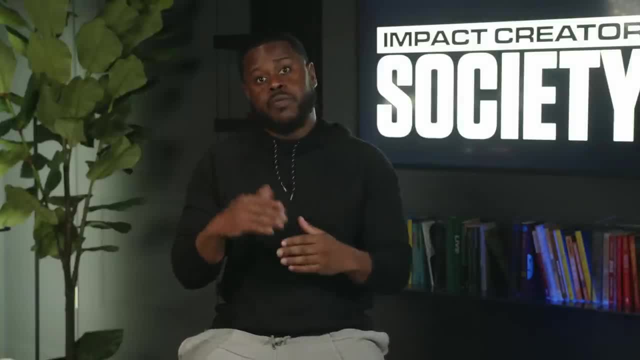 in paycheck to paycheck. When you dive deeper into this study, the study reveals that, out of that, 70% of people- a large portion of those- are people who make over six figures. These are people who are living paycheck to paycheck because of inflation, because of job loss, But a lot of 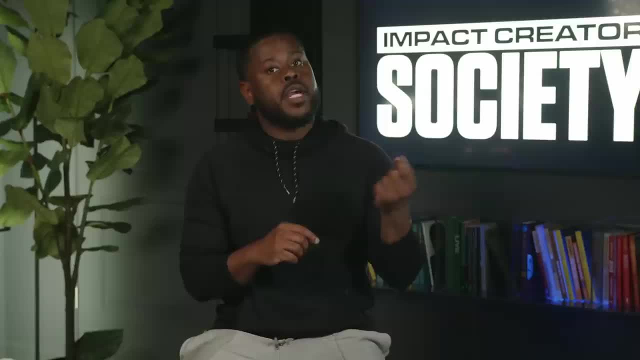 people saying, man, we have an income problem. And here's the truth. We don't really have an income problem. We have a lack of utilizing our gifts and skills problem. You have the skills. you have the talents that God put on inside of you, And I want to ask you this question: Be very 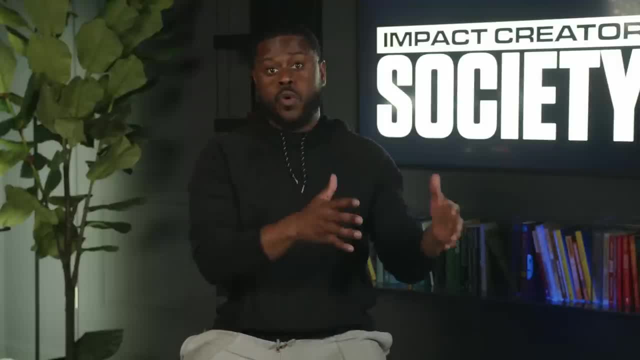 honest. Are you utilizing them correctly? Or are you just going to work getting that check coming back to your gifts and skills to build wealth, to pay off debt? Well, listen, I am hosting a free, a 100% free- masterclass here with the next few days And I'm teaching people how to build a. 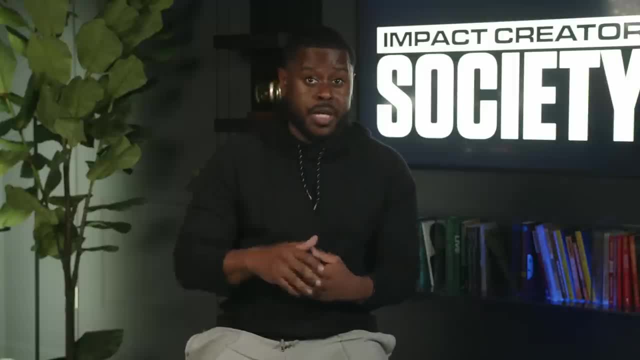 personal brand, how to use the gifts and the skills that God put on the inside of you and turn that into an extra thousand to $5,000 a month to go towards paying off debt, to go towards building an emergency fund, to go towards building a dream home. But I'm going to go even a step. 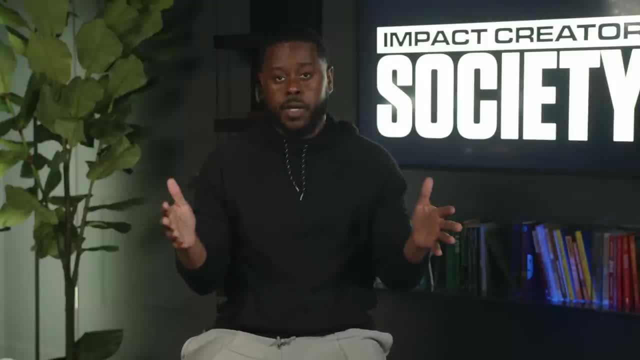 further. What if you can use the same principles I'm going to be teaching for free? You make an extra thousand to $5,000, but what happens if you could turn it into a six-figure income or maybe a seven-figure income within the next couple of years? Well, if you are ready to take control of 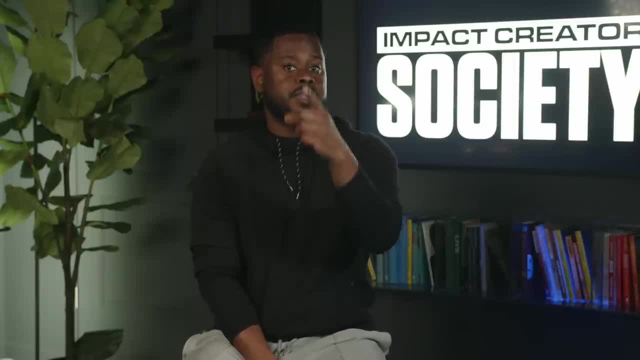 your money if you're ready to utilize the gifts and the skills God has given you to build a legacy, to build wealth for yourself. can you meet me? I want you to go to anthonyonealcom forward slash. save my seat. Again, that is anthonyonealcom forward slash. save my seat Or you can click. 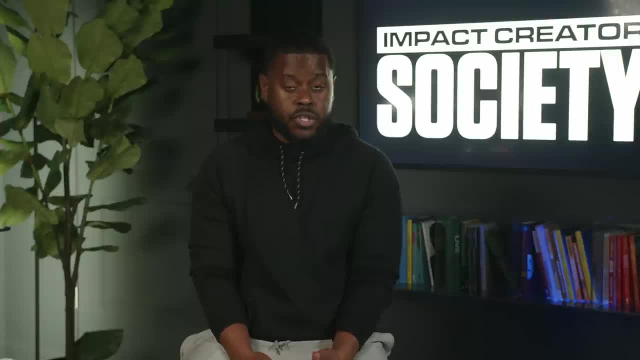 the link in today's show notes. It's 100% free. Come join me, Let me show you. Let me show you how we- my team and I- built a seven-figure brand and how we can put a thousand dollars in your pocket for the next 30 to 60 days. I'll see you soon. While I say that, nowhere is 100%. 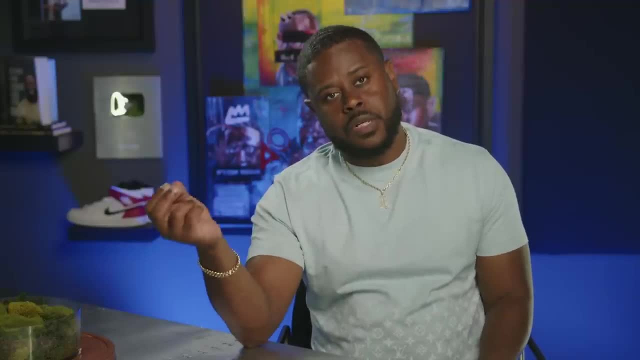 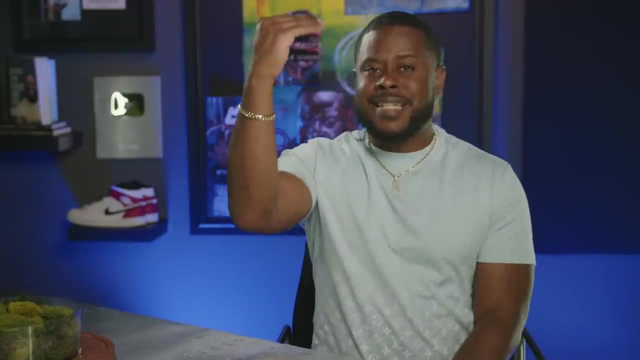 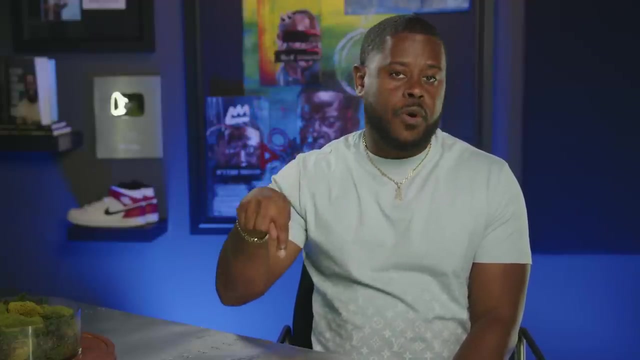 safe. I am not saying: move into the projects, move into the hood if you have the means to go somewhere else. I'm not saying that. But what I am saying is: don't max out your income or don't go above your 25% just so you can save your money. 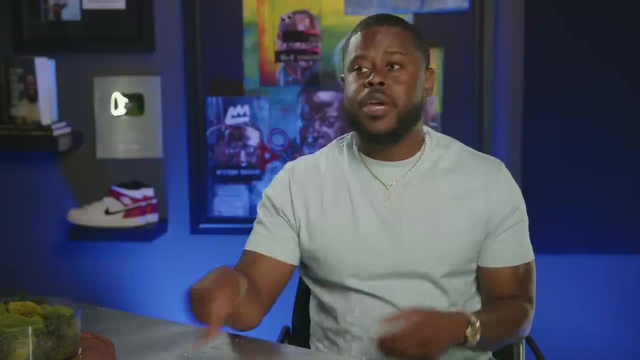 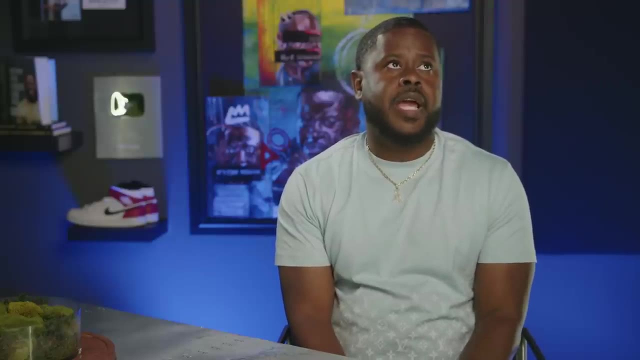 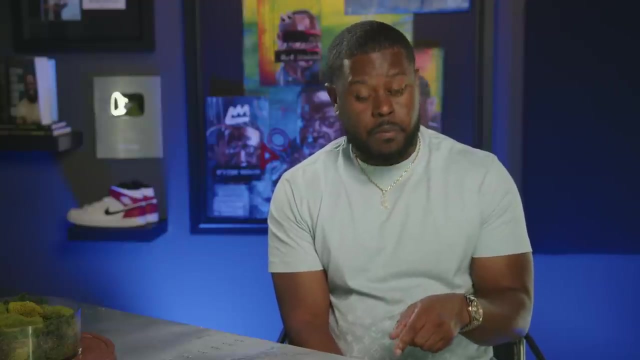 You live in this neighborhood. I make great money. I make great money And I just told myself, no, the bank approved me for a huge loan, for a mortgage, And I said, no, my budget, based upon my budget, is X amount of dollars, because I am not going to go over 25%. 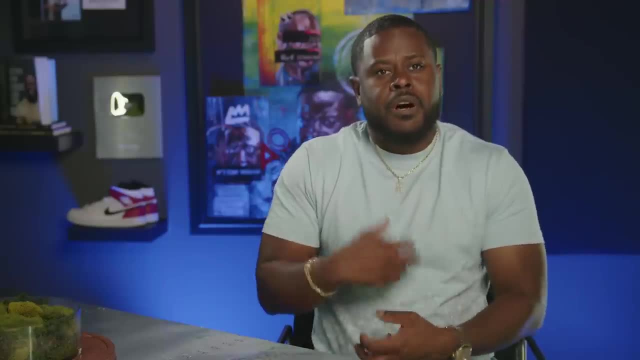 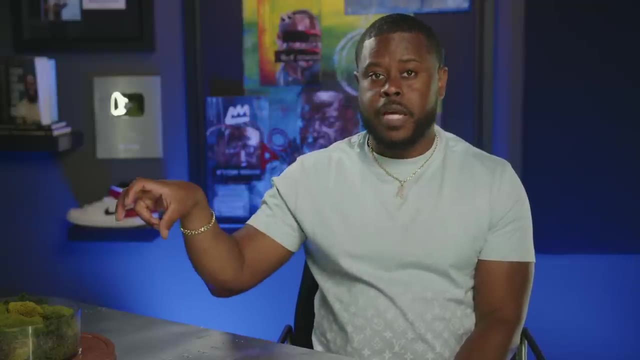 I do not want it, because I love the freedom of doing the things that I want. I want to do, And if I go above 25%, I'm not going to be able to do that. Some of y'all. when your lease is up, you need to move. 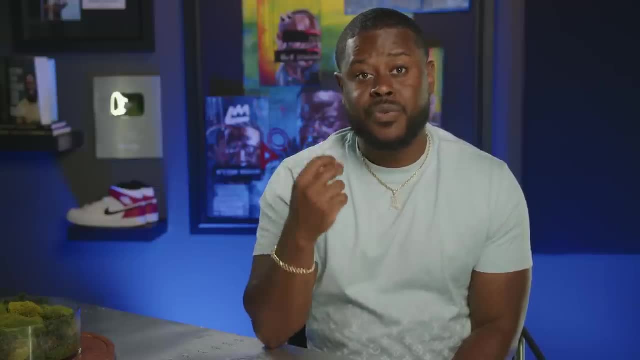 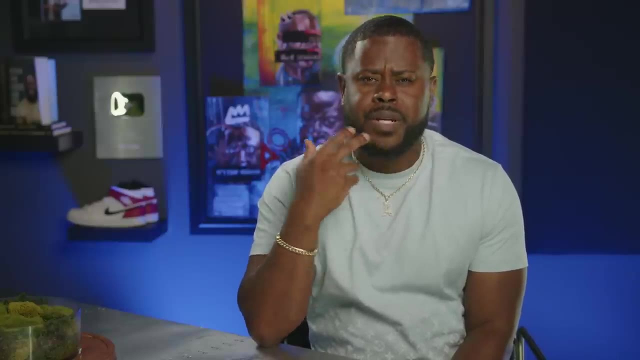 Some of y'all need to go ahead and sell the home because you're stretched, You're frustrated. You and your spouse are arguing not because y'all are mad at each other, because you're stressed with finances And one of the biggest stress factors when it comes to finances. 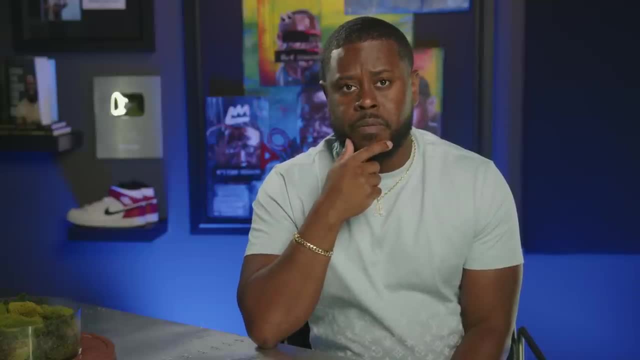 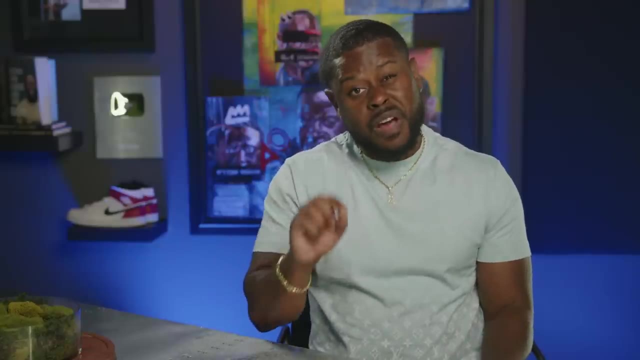 are your mortgage payments? I really want you to sit back and think about it. Are we over 25%? Some of you all are, And if you're over 25%, sit down, look at your budget, have a conversation with your spouse. 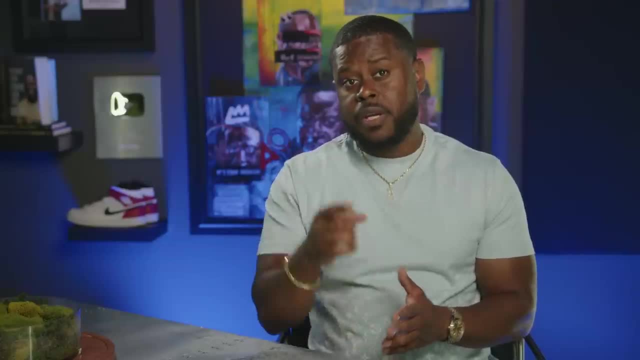 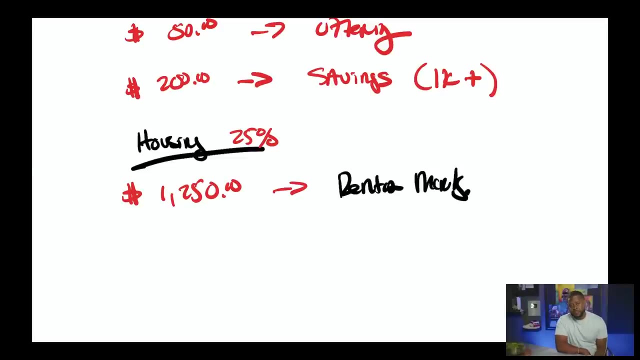 have a conversation with yourself or an accountability partner, if you're single, and identify what can we do to change this. So, now that we've sat down and we said, okay, cool, we have our mortgage payment, we need to sit down and talk about. 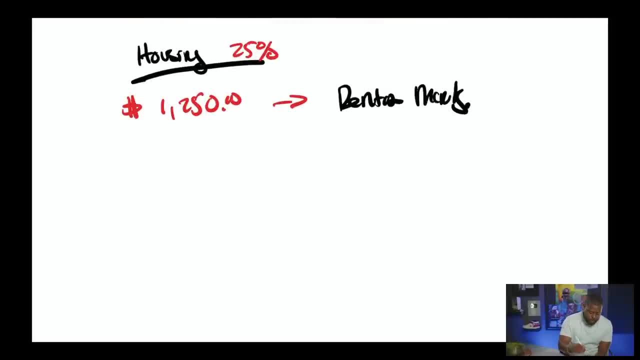 what utilities are we doing? All right, So now, if we have the utilities here at. you got your water bill. I'm spending about a hundred dollars a month on water. I'm gonna go back and change that. I'm spending about a $50 a month on my gas bill. 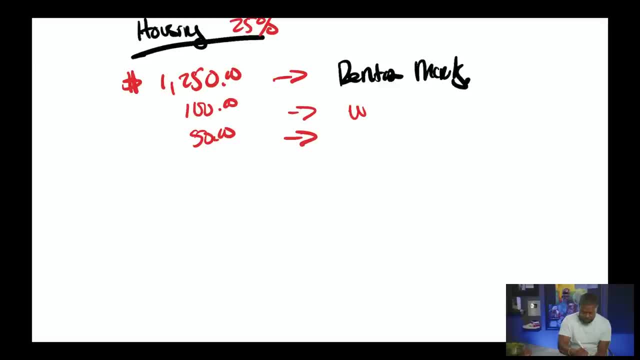 I'm spending about- uh, I'm spending about- on my home, because I work out of my home right now. I'm spending about a hundred and fifty dollars on a cable and internet, And it really is just internet. Just internet for me, right? Just internet for me. I don't have cable. 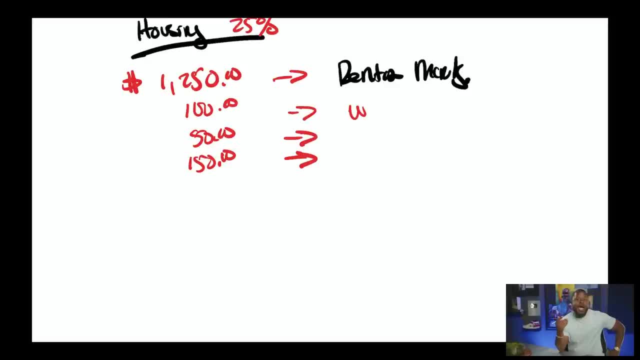 I actually use. I pay for the app through my company. I don't pay for the box. No, no, no, no. I don't do none of that. I don't do. I don't do none of that, All right. 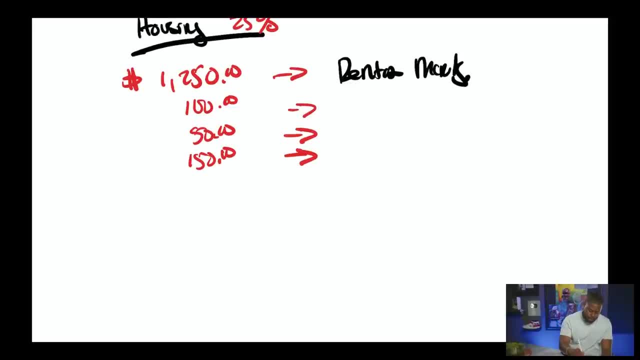 So my, let me go over here, erase this. So this is going to be my. what's this right here, y'all, This is gonna be my water bill. I didn't change that over to black. This is going to be my water bill. This is going to be my gas bill. 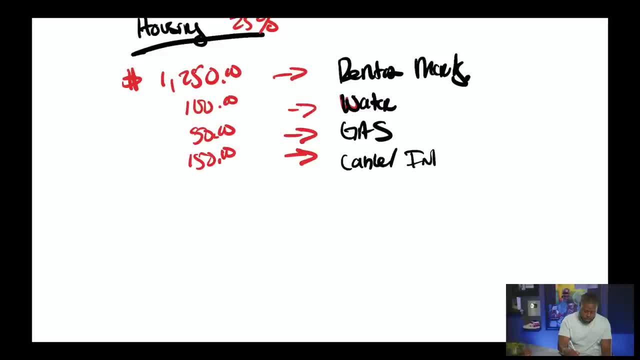 this is going to be my cable and internet. Okay, Then you know what We have to add in my electricity. My writing sucks, but I love it Electric, So we have on electric. I'm spending, depending on the summer months, I could be anywhere from $300 to $400 because I have a pretty nice size home But then during the heat, during the winter months, I mean I'm not even running it and I don't even run my heat. So I say, on average I'm spending about $200 a month on electricity. All right, $200 a month on electricity. I'm estimating that because high. months for the heat. for the summer I love my house to be at right around 68 to 70. Don't judge me. But then also during the winter months I'm spending about $200 a month on electricity. During the winter months, man, I may be spending $50 a month because I'm not running any heat at. 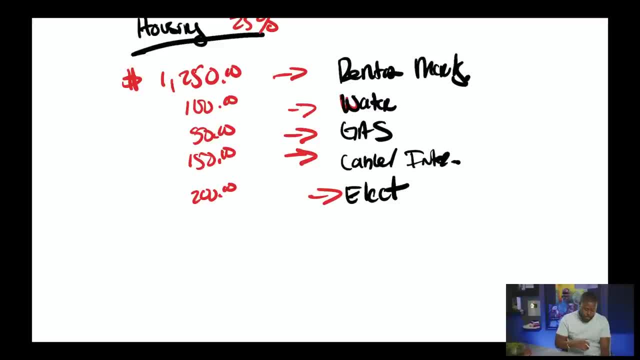 all, All right, And so that's that. So, right, there, we have the housing. Then let's go down in transportation. If I am in this person's shoes, I do not have a mortgage payment. I'm not a mortgage payment. a car note, but that's fine, I am going to put down on average we're spending. about what. Let's just say we're spending about, on average, about $200 a month On gas for the car I'm going to put a gas car, Y'all know what I mean there- And then for maintenance I'm not really. I don't think too many people are spending that much money on. 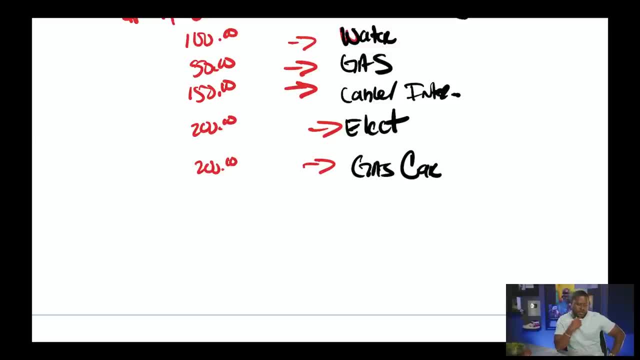 maintenance. You got oil changes, what every three months? or every five, 10,000 miles. So let's just say, right there you're setting aside, let's say $50 a month for your gas, right? Not your gas for your maintenance. 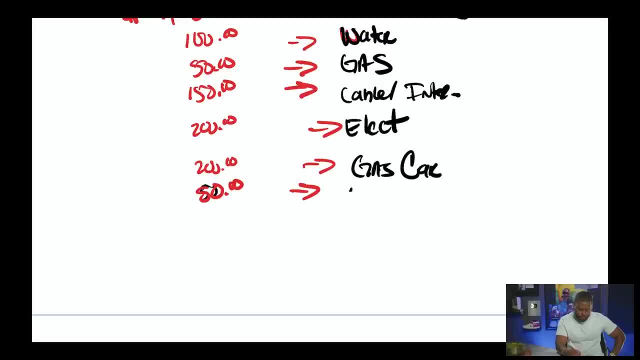 Maintenance, All right. So let's just say, for oil change, Okay, For oil change, All right. So then from there, boom, we're going to keep on going. Then for groceries. Now, this is where some of y'all mess up at, This is where some of y'all mess up, right here. Let me tell y'all right. 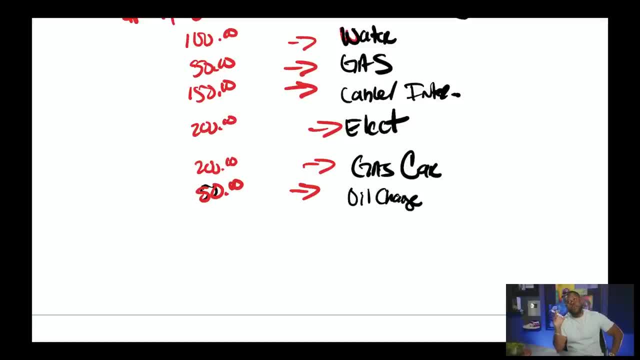 now Some of y'all are spending way too much money on groceries. I'm a single man who eats a lot. I got to eat three good, solid meals a day because of my food regimen, plus some snacks. I'm only spending about $180 a month on groceries. Now I'm spending that because I'm actually buying. I'm buying higher quality healthy stuff. Let's be real: Some of y'all- you probably can get upset when I say this- Some of y'all are not eating healthy, So you don't have to spend $180.. I'm buying fish, I'm buying high protein chicken and I'm buying from from from the fresh mart. 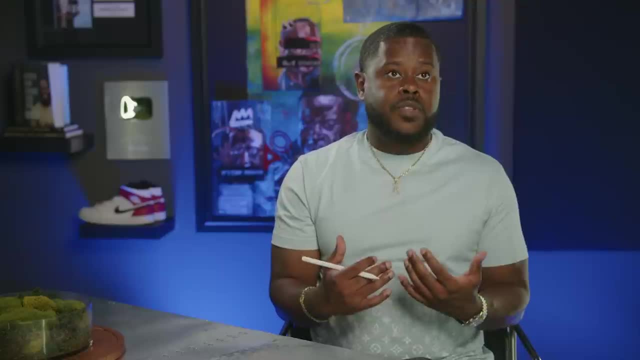 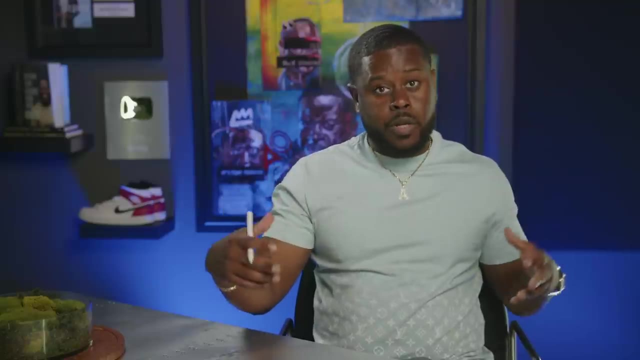 right. So that stuff is expensive. but I'm also buying in bulk. So that way I'm not just buying one piece of fish, a custom. I'm going to the boat places and I'm getting boat fish, boat chicken, I'm grilling it, I'm putting it on my smoker. You know, I'm buying some. 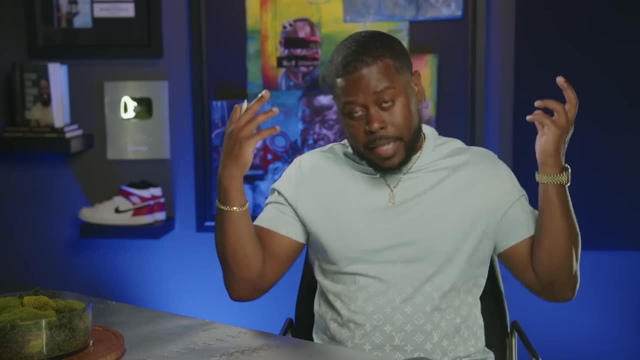 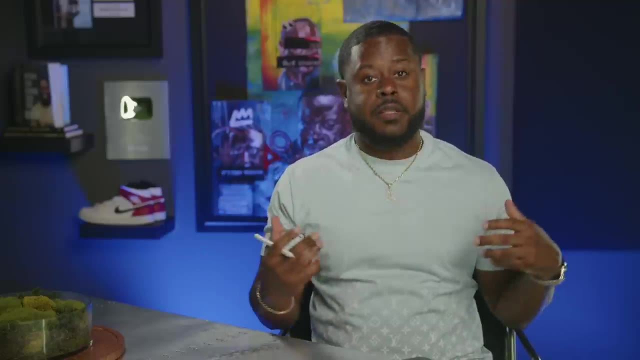 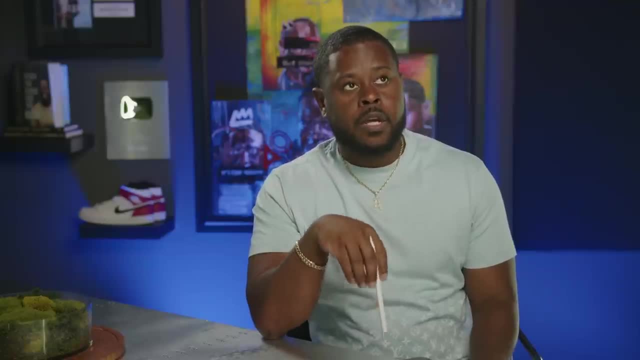 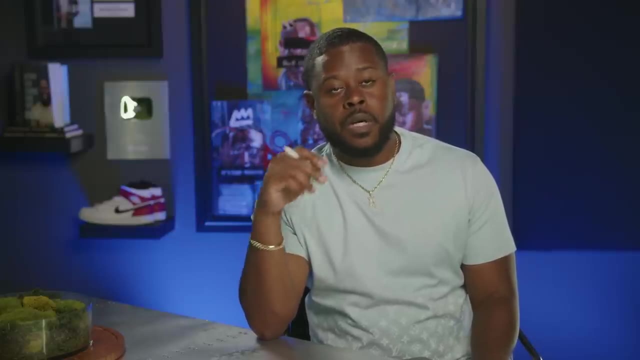 And what you buy, which is someone wants to eat right now, but you're not thinking about the future of. okay, When I get home, how am I going to make a meal I don't know about? some of y'all put it. drop it in a chat. Let me know. if you're on podcast again, come over to YouTube. 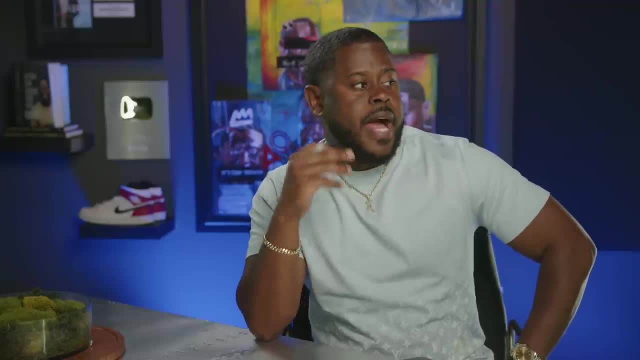 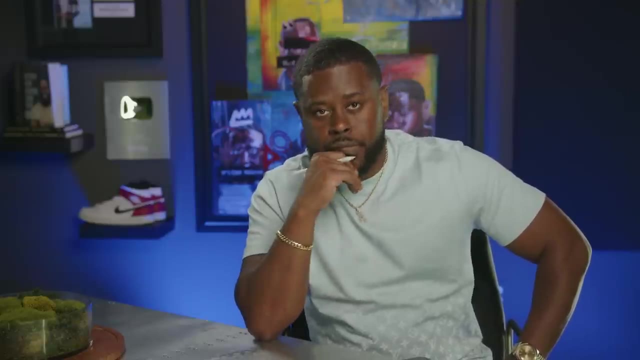 drop in a chat or come over to my Instagram channel, drop me a DM. But how many of you all spent $150 on groceries, get home and realize you didn't buy anything that you can make into a meal? I've been there several times. I've been there several times. I've been there several times. 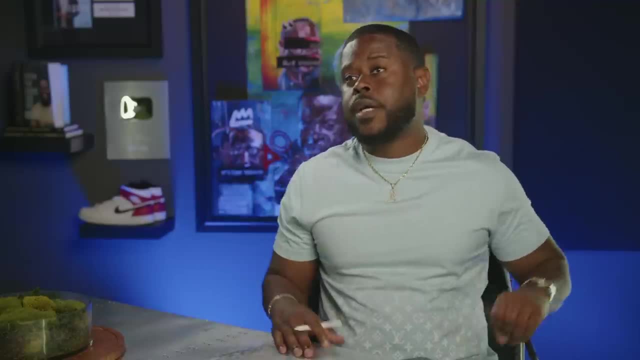 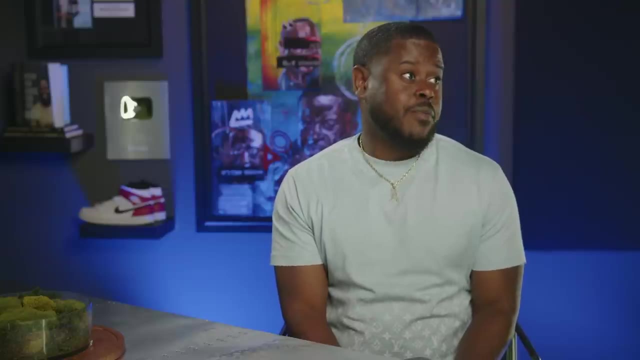 Because I went when I was hungry. I bought chips, I bought crackers, I bought this, I bought that. But when I got home and I unpacked everything, I didn't put nothing in my freezer. I didn't really put nothing in my refrigerator, but some drinks. everything was going to my cabinet, a bunch of 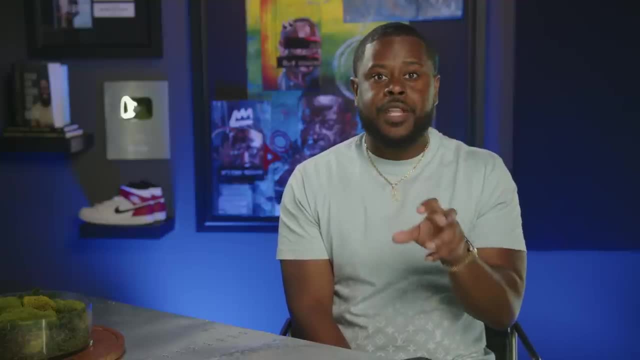 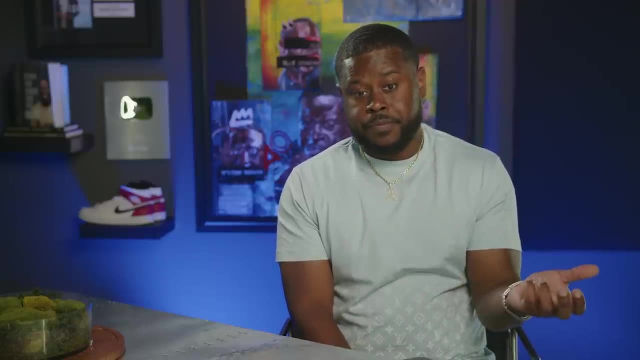 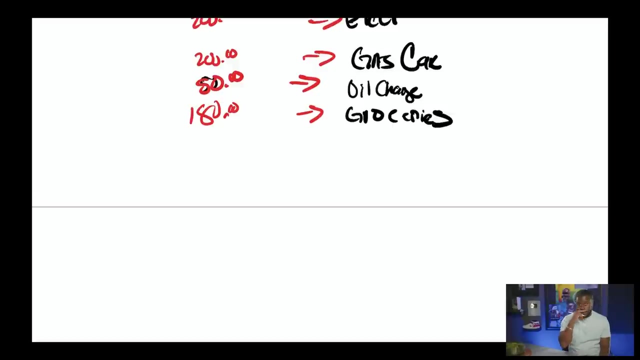 snacks, a bunch of this and that that it really wasn't anything good for us to make for a meal, So we got $180.. On groceries: cell phone bill, I use Verizon. I rock with Verizon. I'm spending a hundred dollars a month for my Verizon bill. 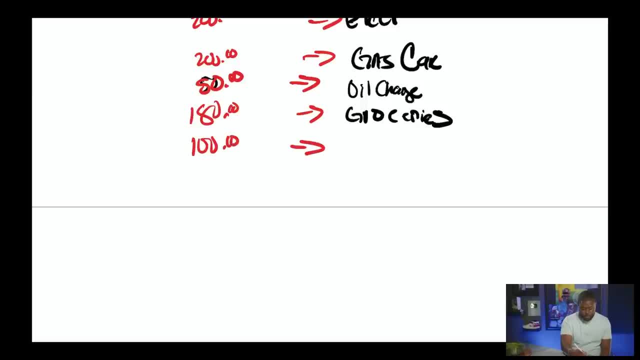 If y'all know anybody who's better than Verizon, please let me know. I will switch over today. I need a cheaper bill. As a matter of fact, anybody who wants to sponsor my show and you got a good cell phone service, holler at your boy, Cause I need a cheaper, cheaper, cheaper bill. 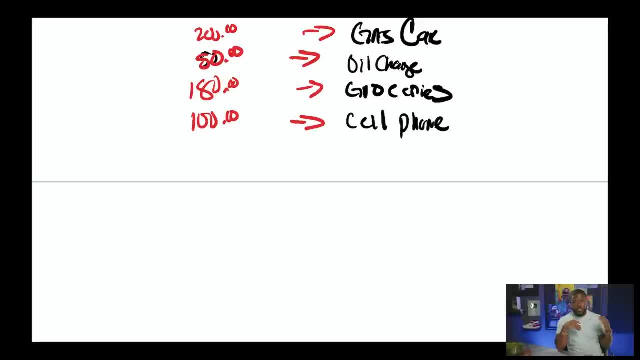 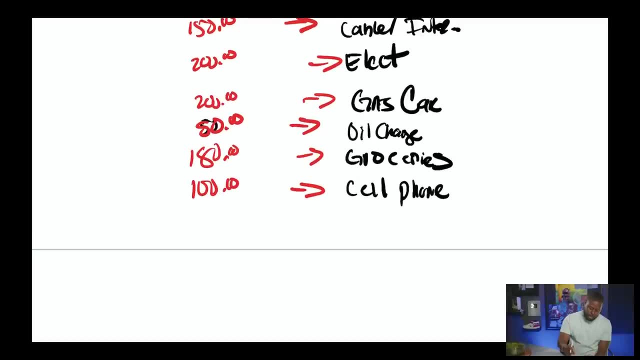 on your every dollar app. Two, And when you're doing a zero base budget, watch this, you guys: after you list that, after you list your cell phone and your, your, uh, your- cable bill, you got to list your. 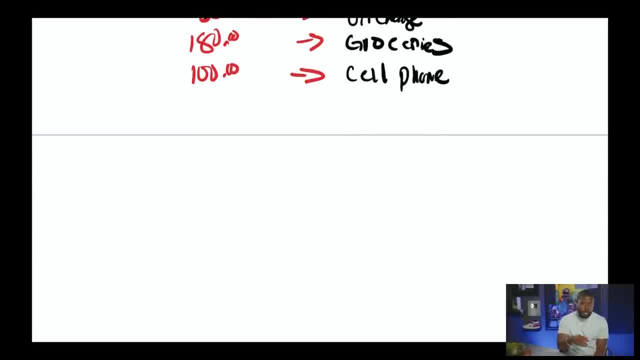 subscriptions. I'm probably spending right now a month, honestly, about $50 a month on subscriptions. I'm just going to put subs. I actually need to change that color So y'all can know that I'm only spending $50 a month on subs. 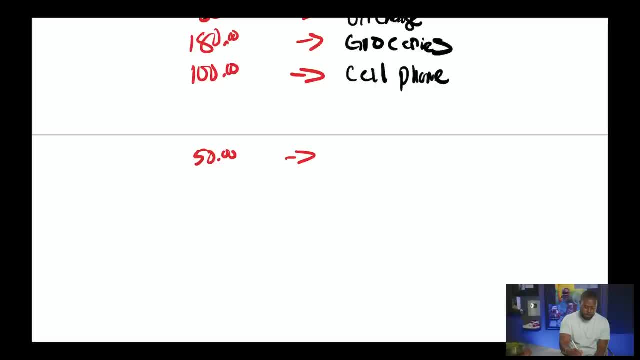 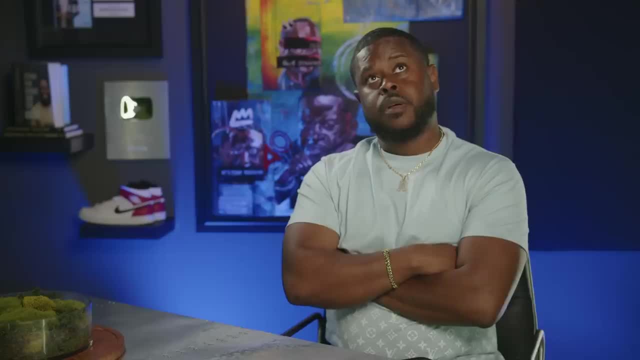 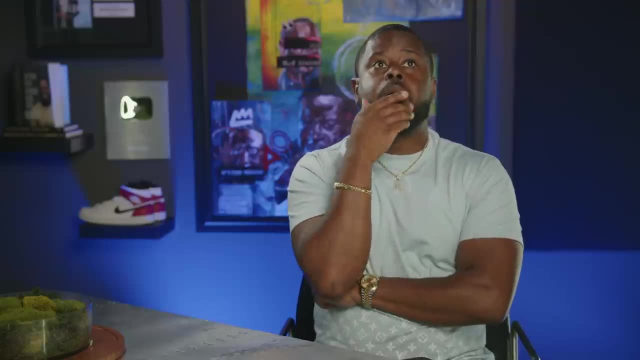 How many of y'all are spending more than $50 a month. Drop it in the comments and let me know if you're spending more than $50 a month on subscriptions, How much, how much, how much. I can tell you right now. some of y'all are probably spending about. 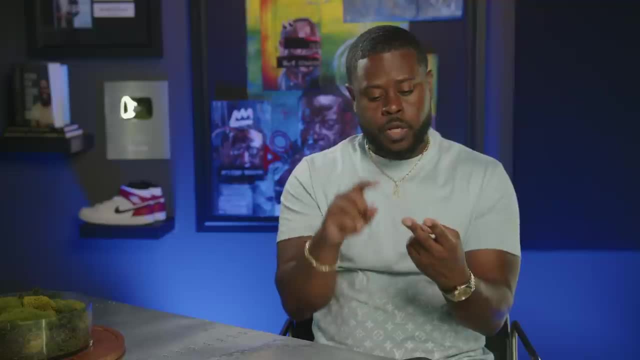 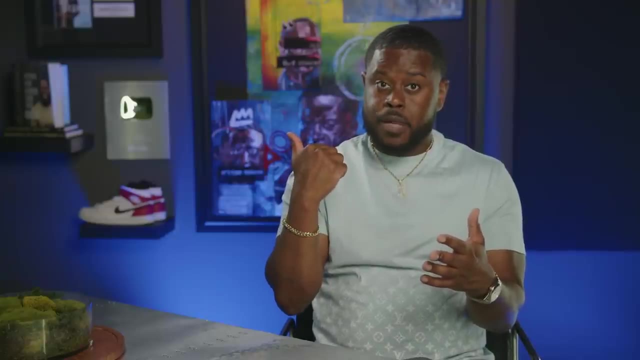 $200 a month. It's just on subscriptions. You got Hulu, you got Netflix, Amazon, prime, HBO, max, center, max, Disney, plus brain Keep going. Some of you all got Spotify, Some of y'all got Amazon, Some of y'all paying for Pandora. 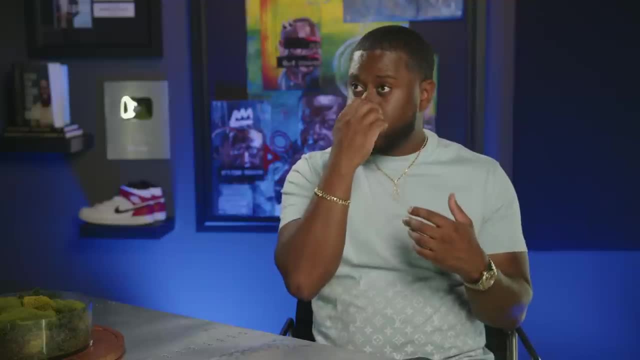 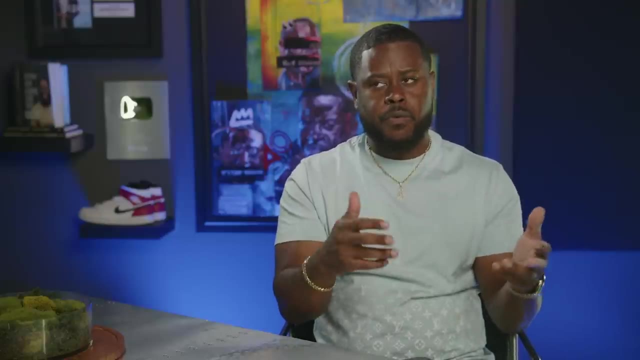 Some of y'all paying for satellite XM radio. It makes no sense to me. Why are you paying for satellite XM radio When you're going to plug in your phone to get Apple car play and you're going to open up your Spotify, your Apple music, to pay for it? Why are you listening? 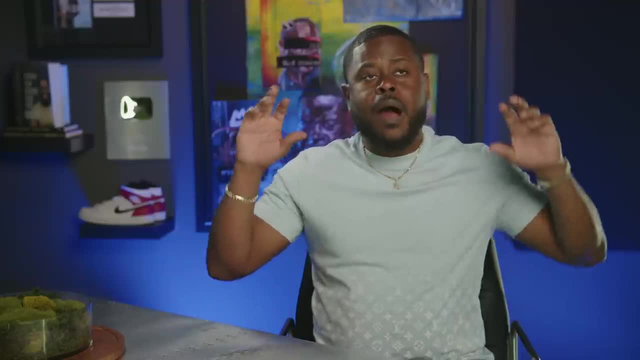 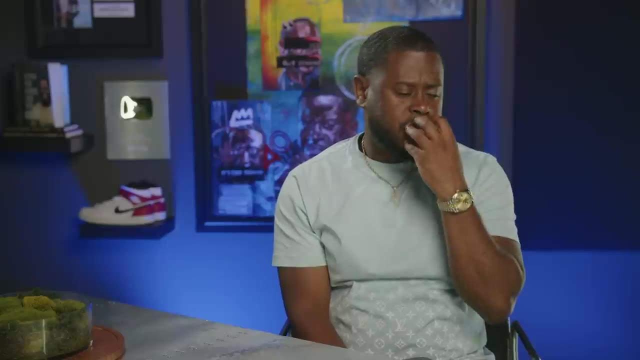 to XM radio. Why are we spending all these money on apps? Some of y'all have about five different apps. that makes you look good. It makes your smile look a little bit better. Make sure your smile. you can fix your teeth. make your teeth. 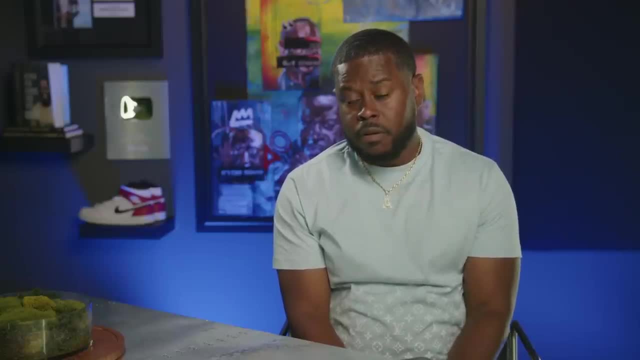 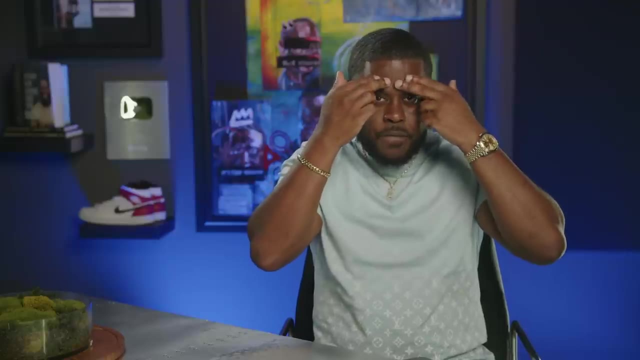 Right, When you know the yellow huh, You make your smile a little bit smaller but more polite. You get all your blemishes off of your face Like y'all got apps for everything because you're trying to get your likes. 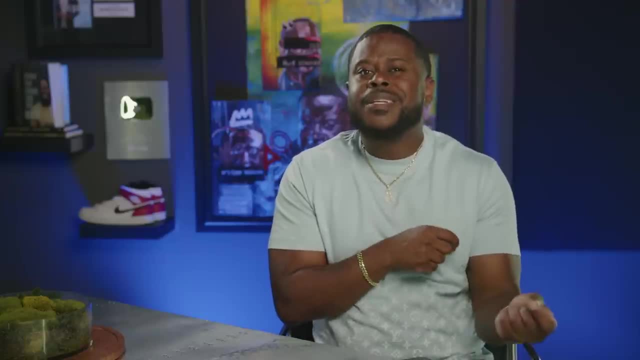 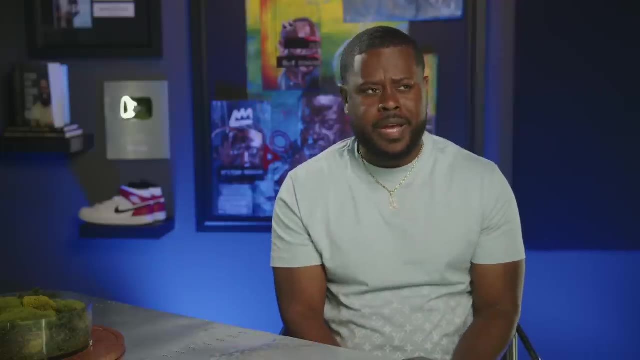 If people don't like you for who you are, you are in the wrong place. You're around the wrong people. If people don't want to rock me because I got a dimple in the middle of my forehead, bye, I'm not going to get rid of my. 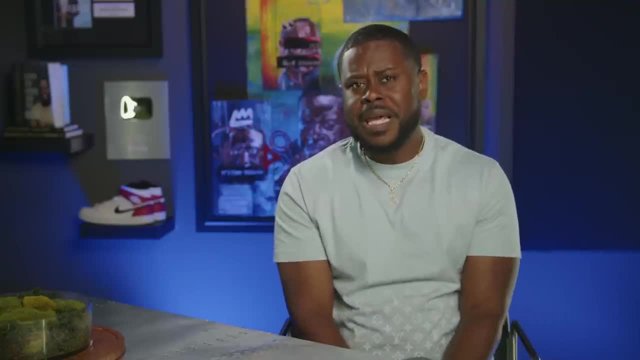 dimple on the internet. I'm going to get rid of my dimple on the internet So that you can see it in person. No, it's misleading, but you're paying money to make yourself look good When you're already a beautiful or a handsome individual. 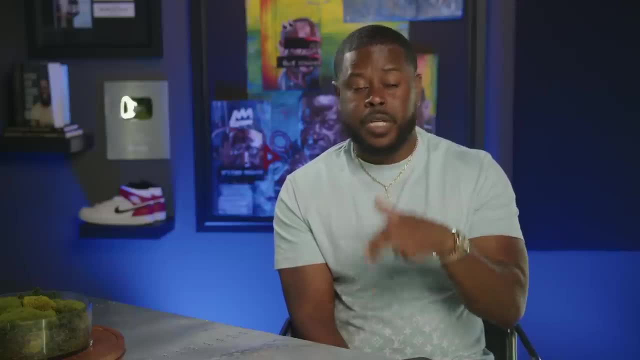 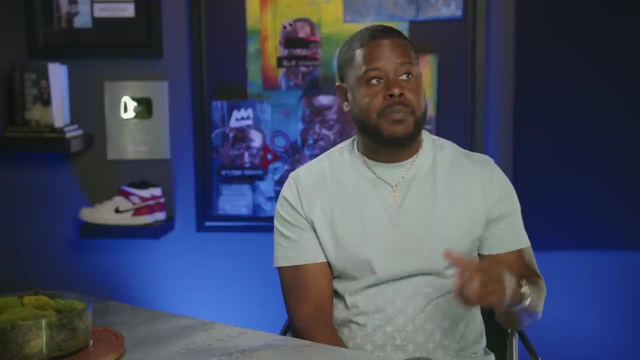 You got to list all of your subscriptions on this budget. And here's the truth. You guys, you all may list all this stuff And at the end of the day, you all may come up and be like, oh shoot, I'm overspending And I'm about to show you. right now I'm not even adding up this stuff. 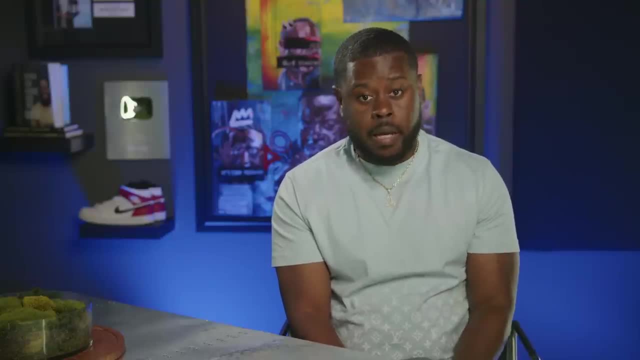 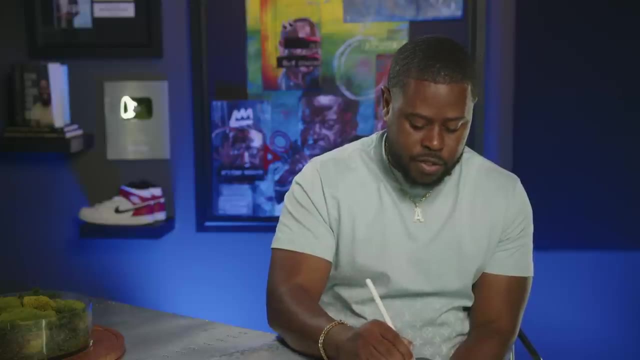 I'm not even calculating this stuff. I don't know where we are right now, but we're about to add it all the way up. Some of y'all ladies are spending y'all about to get upset, but I already know some of y'all spending $500 a month just on your hair. 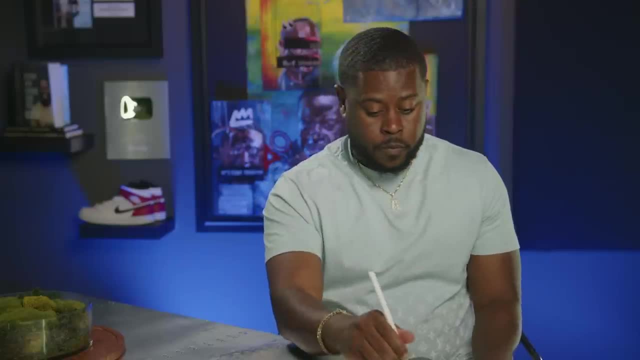 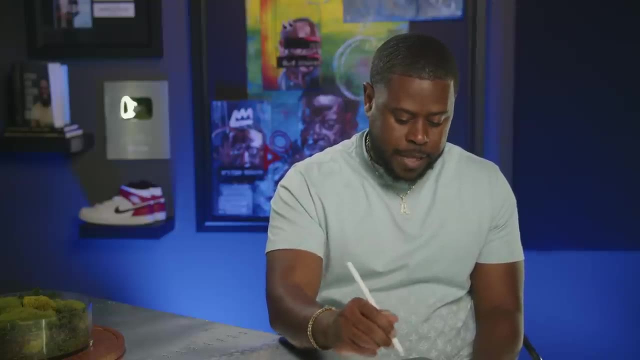 Just on your hair. I know that for a fact, some of y'all spending that much money on your hair. I know that for a fact, Y'all buying weave, y'all buying wigs, Y'all got to pay the person to put. 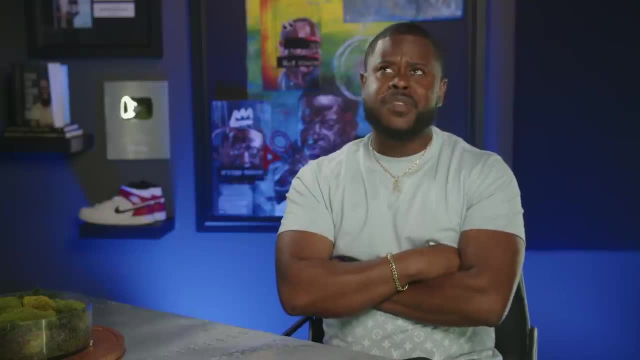 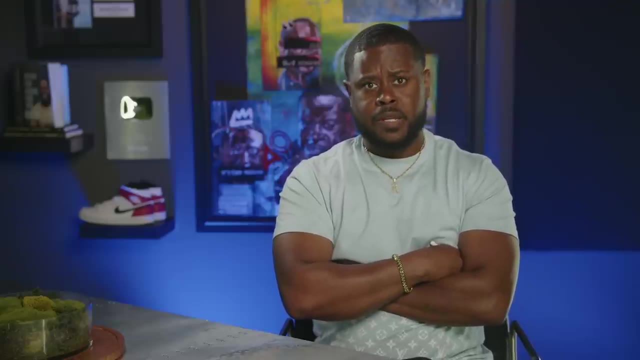 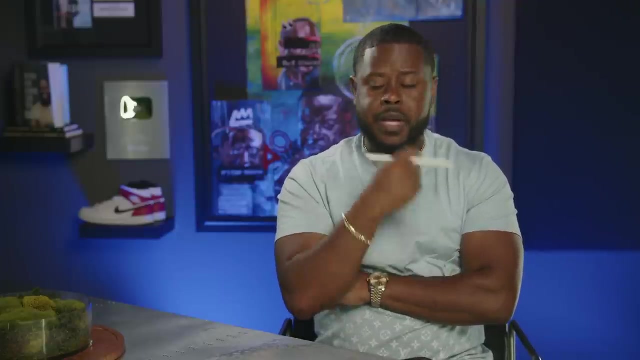 it in. I know someone right now. she spends about two grand a month on her hair. I'm like: what in the world? What are you doing? This is ridiculous. You can't work for me. You spending two grand a month on your hair? I don't want you working for me. That's just crazy. That's just crazy Brothers. what are we spending? I'm spending $200 a month on my haircuts. I pay $50 to get a haircut every week. $200 a month. Girls out here spending two grand a grand $500.. You got to list that on there too. 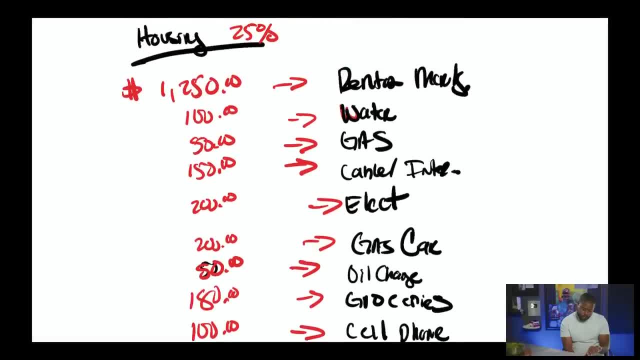 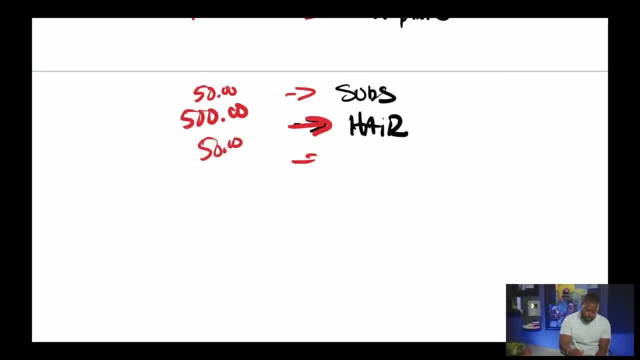 You got to list it on there too. Did I list my for my groceries? I did not. So for my dog, I'm spending about $50 a month for my dog food. Okay, That's dog food, All right, Then from there we're going to come down here and we're going to list all of our 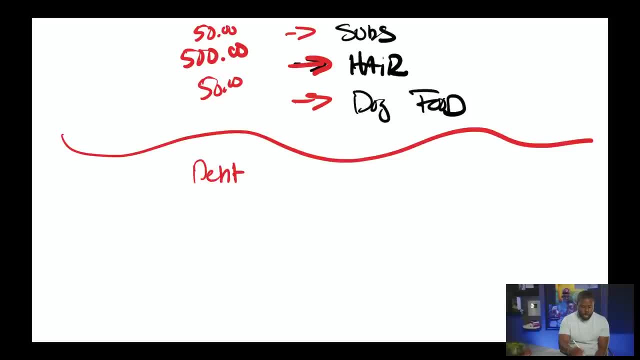 debt. Some of y'all have a car note. $700 for the car note, Jesus, Jesus, Okay, Some of y'all are spending about $500 a month on student loans, Jesus, And I believe it. right there, All right. So let's add all this up. 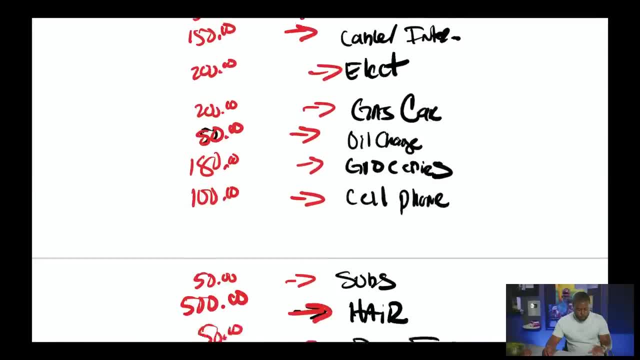 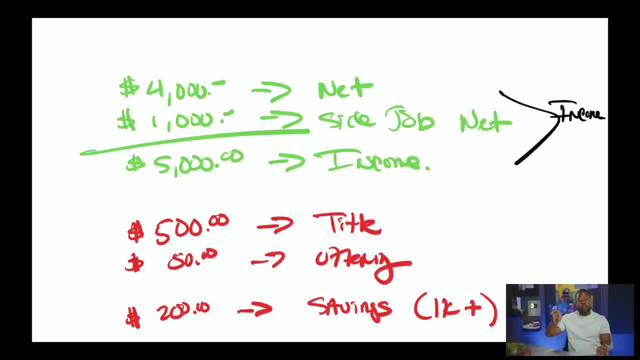 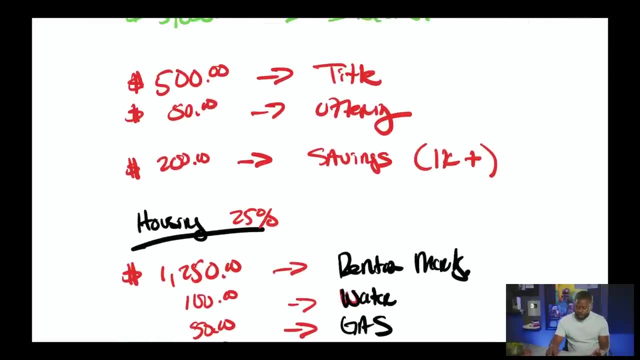 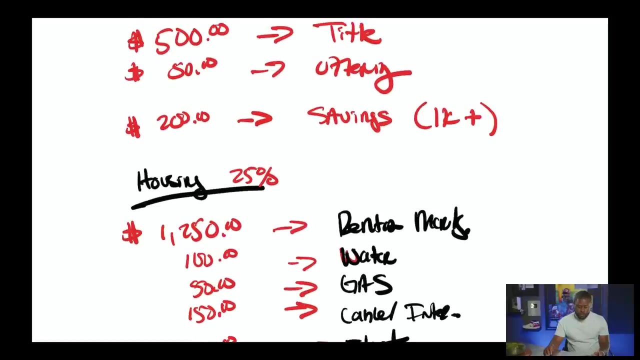 Because remember, um, remember, this is all about spending all $5,000 of this on paper before the month begins, So you can see exactly where you are. So if you are giving away $500 to your local church and giving away another $50, that puts you at five, 50 plus, you're giving, you're giving. 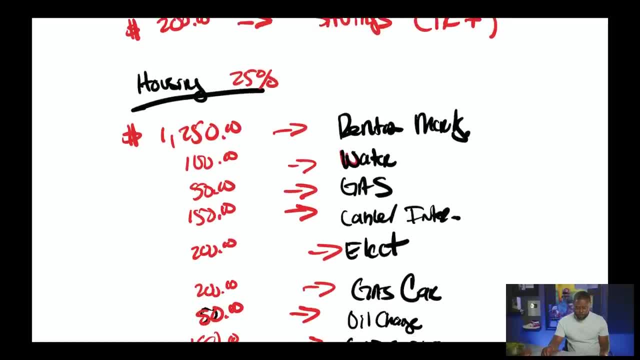 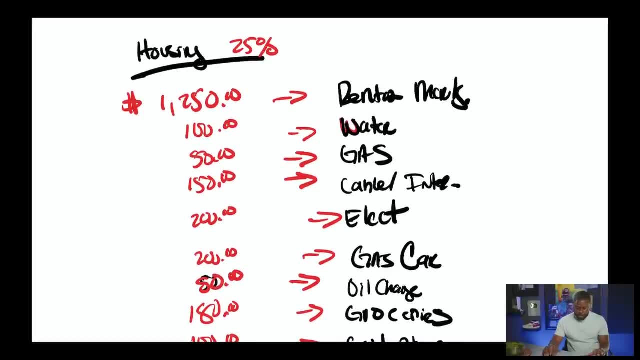 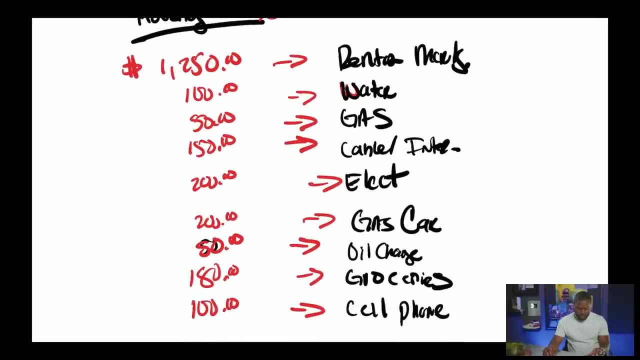 yourself another $200 into your savings. You're at seven: 50. Then we had, when we added our housing and our living expenses, $1,250 for our mortgage or rent payment. another a hundred dollars there for a water bill, $50 for our gas, $150 for um our cable and internet, $200 for our electricity. $200 for gas, uh, $50 for our oil changes and car maintenance. Then we got $180 for our grocery bills And we have a hundred dollars for our cell phone. that puts us at $3,030.. Then we come down here, we add another $50 for our subscription plans, another $500 for our hair. 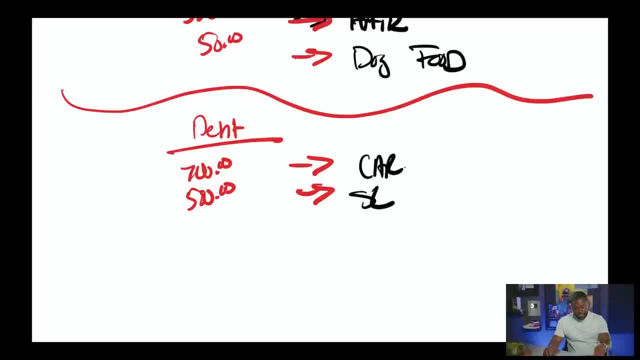 Then we have another $50 for our dog food. We're at 3630 already. And then let's just say we have a car payment of $700. That's $4,330.. And we have another $500 for our student loans. We're at 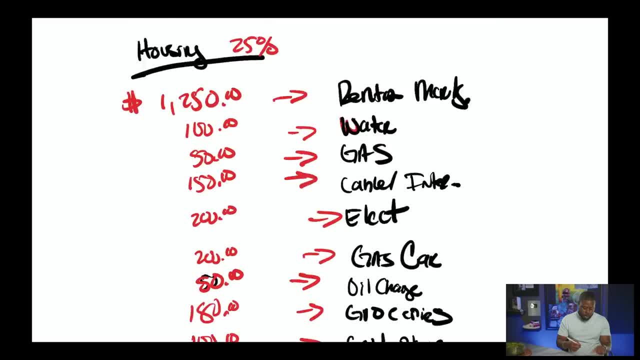 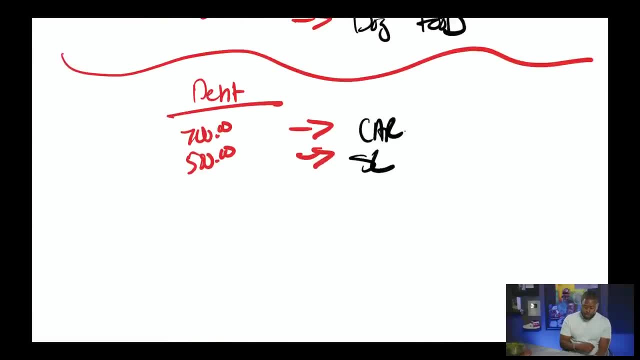 $4,830, right? So already we are close to our $5,000. and check this out, You guys. we didn't even talk about car insurance. So let's just say we're spending right now on average. Uh, let's say we're spending a hundred dollars on car insurance, right? So what does that put us at? 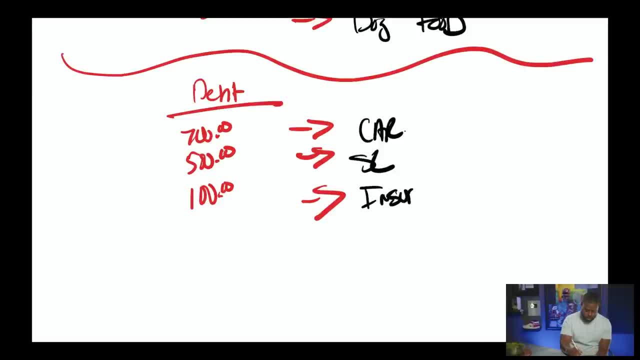 Let's put that in insurance. Okay, Okay, That puts us at $4,930.. So we are at- give me an example here: If we are at a total of $4,930, that means out of the $5,000 that we have to spend, because that is our net pay. 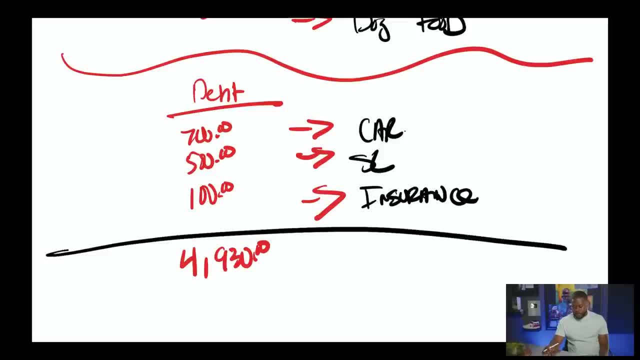 net pay, we have 5,000.. I should be doing my math right here for y'all. Uh, we have $70 left on paper that we need to spend. So if this was the case- and I am that person, I'm spending that $70 on myself. You can bring. 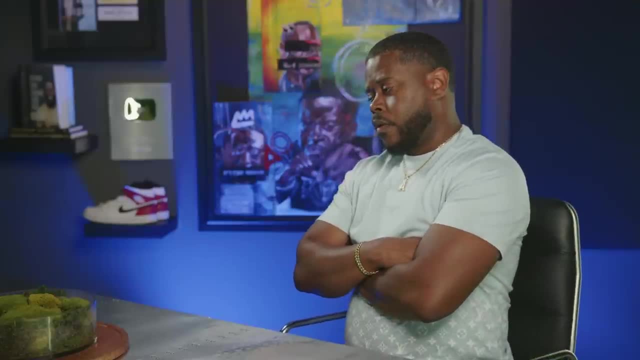 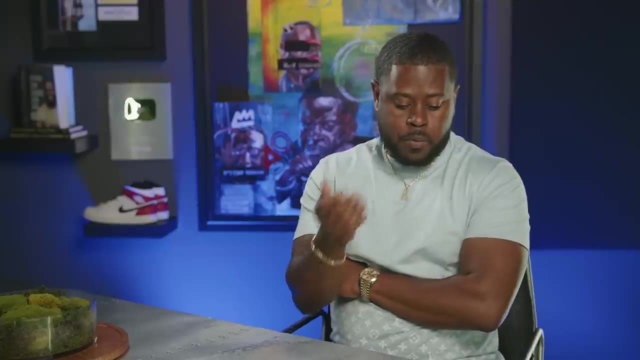 it back to me. Well, having a zero base budget, that's exactly what you do. Let's just say, for an example, we came up and we had $5,400 that we spent on paper, but then we know we have to go. 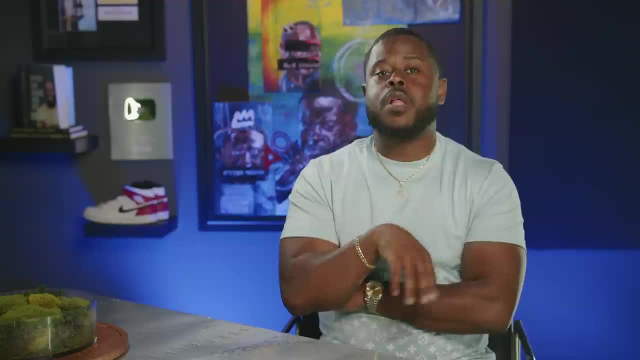 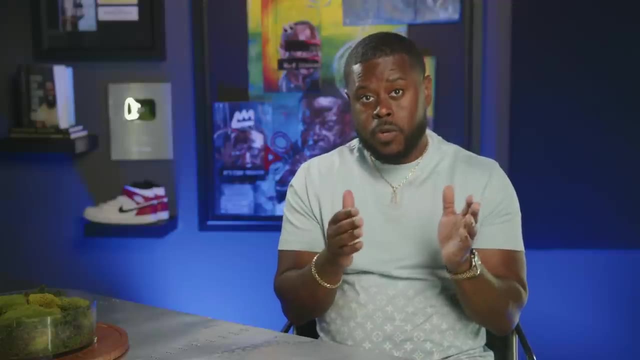 back to our budget and remove $400 from our budget. Some of us will go back to the budget And because we are already so anal, because we're already spending every dollar we possibly can, you may not have a million and one subscriptions. 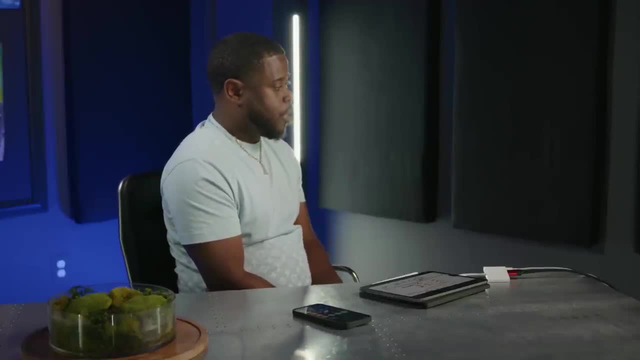 You may not have somewhere else that you can actually, uh, cut back from. The majority of us watching this can and should be cutting back. As a matter of fact, this is what I want you to. this is what I want you to do. This is what I want you to do. I just thought about this off. 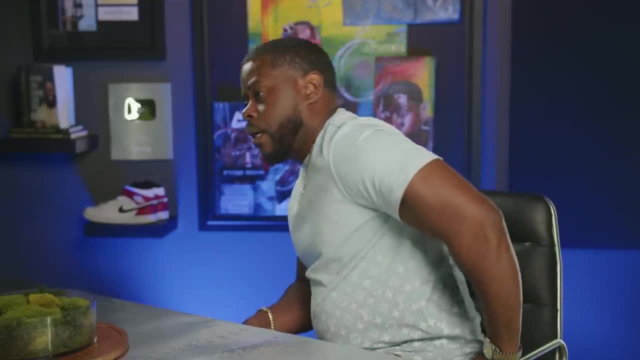 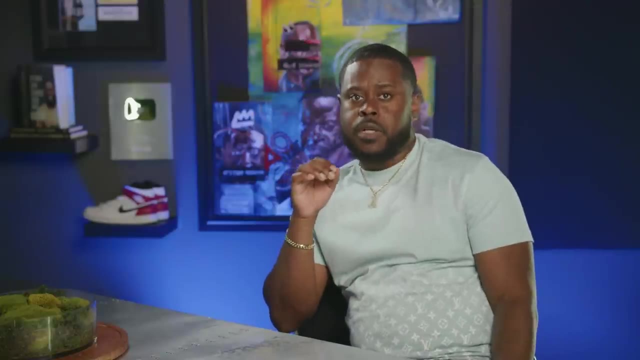 the top of my head, Didn't even tell my team this. This is exactly what, um, I want you, uh, to do If you, if you want to come on my show and get a money makeover, to where you're willing to. 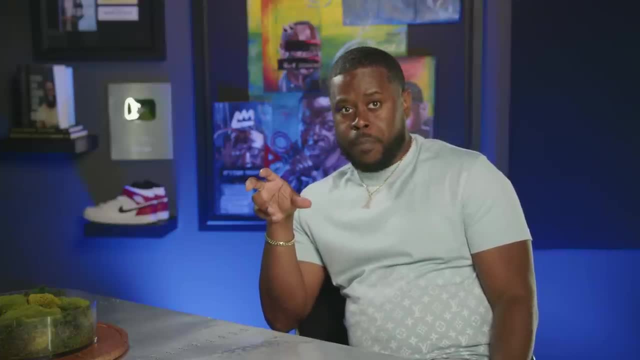 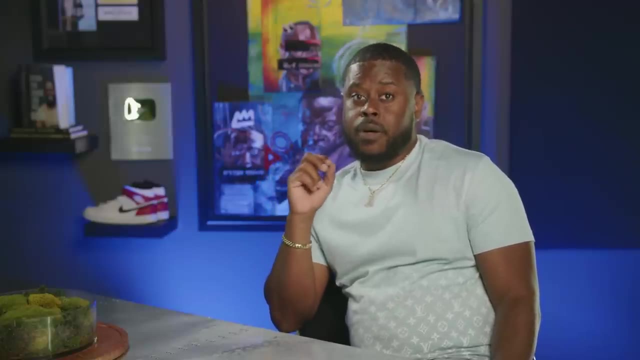 come on a show, sit down with me and we open up your bank account. Uh, you tell me all of your debt and we sit down. you tell me all of your income and we sit down and I answer your money questions and we make a proven budget for you to follow for 90 days. I want you to go to my 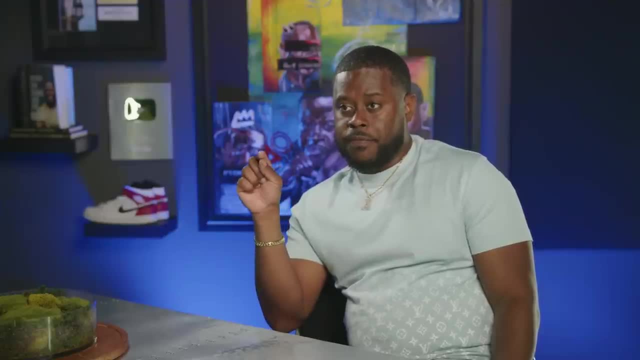 website. go to anthonyonealcom. Forward slash. I'm thinking in my head: what do we want to call this? I'm literally making this up on the spot. I'm gonna have my team, uh, put this form up literally right now, because I want. 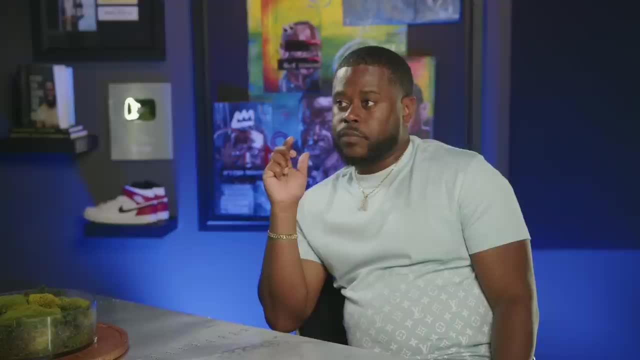 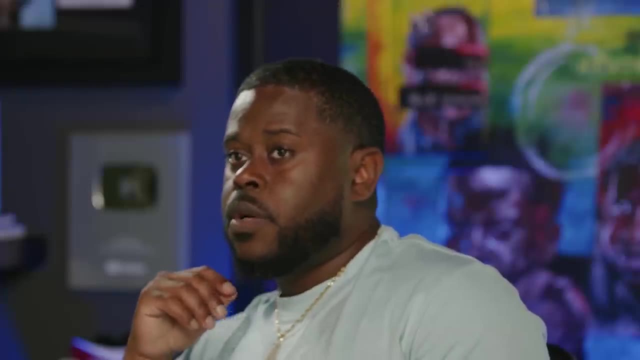 to get some of you all um on the show. That's that's. that's it. That's exactly that's exactly what we're going to do. Go to anthonyonealcom forward slash money makeover. anthonyonealcom. 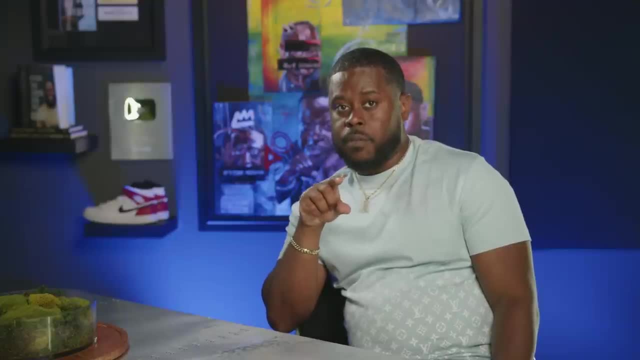 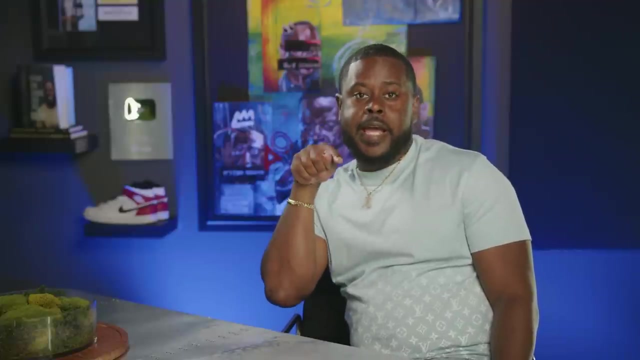 forward: slash money, Makeover. fill out that form. You have to be willing to come on, come here to the table. You have to be transparent and honest. Of course, we're not going to put your personal information out there, but we are going to help people get on a clear, zero base budget. help you understand. 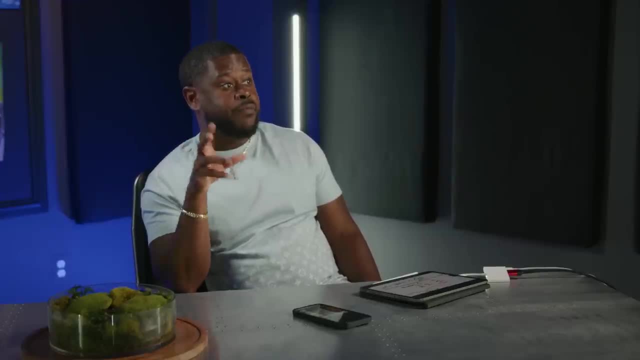 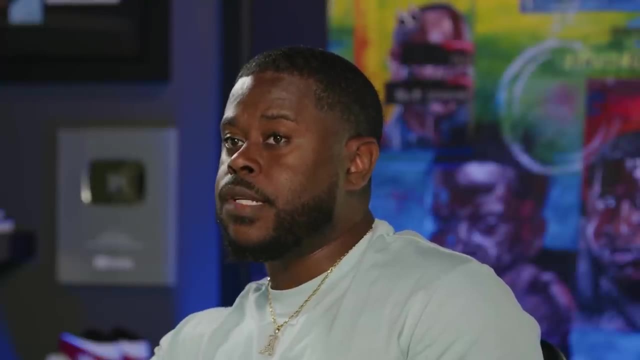 and look at your money, And some of y'all may not like it, but I promise you, if you're willing to sit down with me at the table and help- and allow me to help you with your- your finances- by this time next year you will not be in the same place. Go to anthonyonealcom. 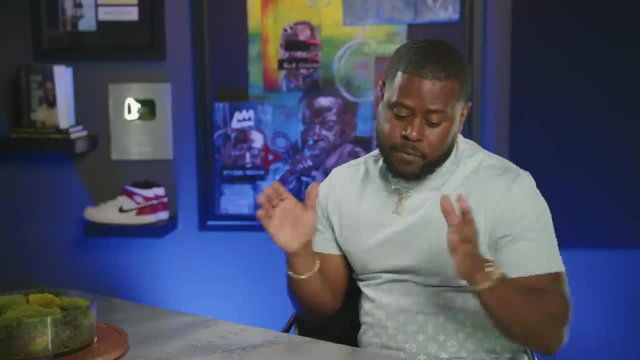 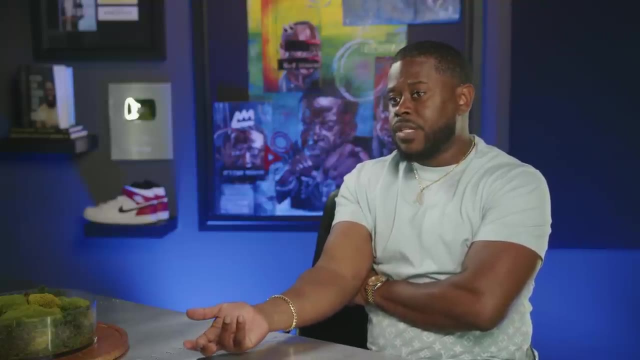 forward, slash money makeover, And we're going to see, we're going to have our team select two or three people. We may even do this once a month, I don't know. We may just do this once a month and just have y'all come over and we just help you out. because here's the thing, Don't be ashamed. 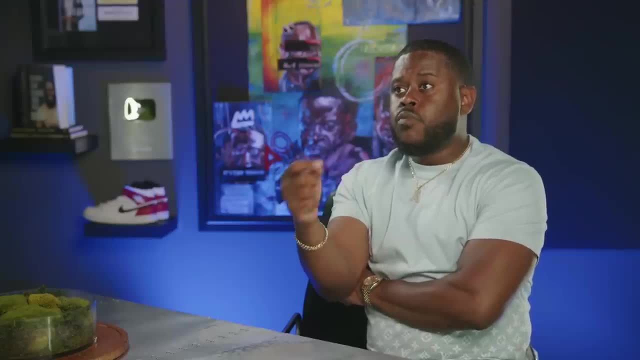 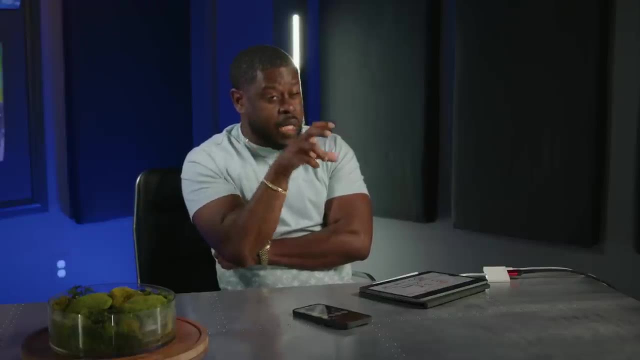 to come over here and get the help, because you may represent thousands of people out there who are scared. But if you're serious about really, really, really changing your life, changing your financial situation and your financial career, go to anthonyonealcom forward, slash money makeover And we're going to bring you on to the 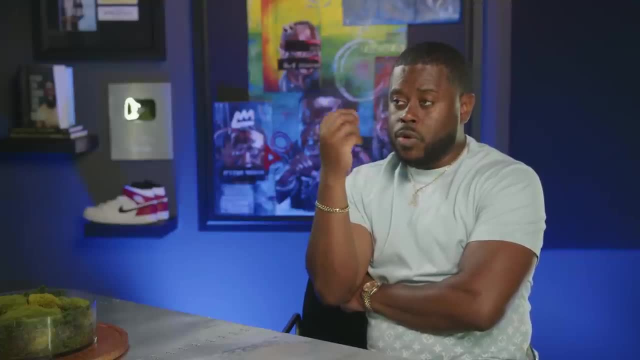 show. Well, I can't say we're going to bring everybody on to the show, but we're going to reach out to people and we're going to help you. We're going to put a proven system in front of you. We're going to help you with your makeover. I was, as I'm ending the show, I was sitting down. 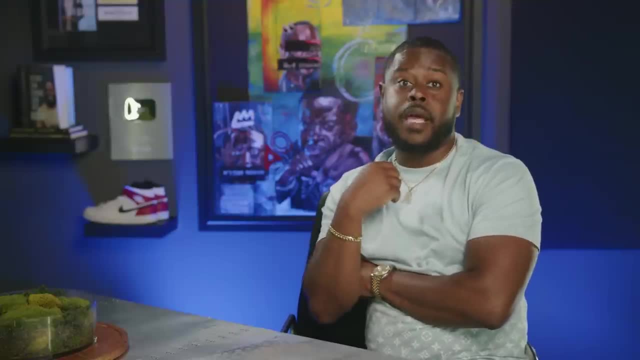 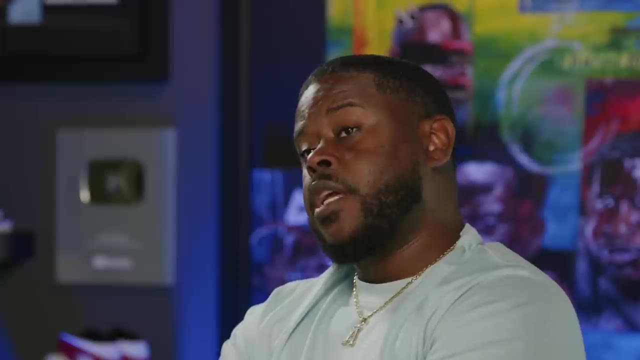 with a guy and I asked him: can I share? He just said: please don't share my name and where I'm in front, So people, people can't pinpoint me. And he said this one thing He said. he said, man, can you help me out my 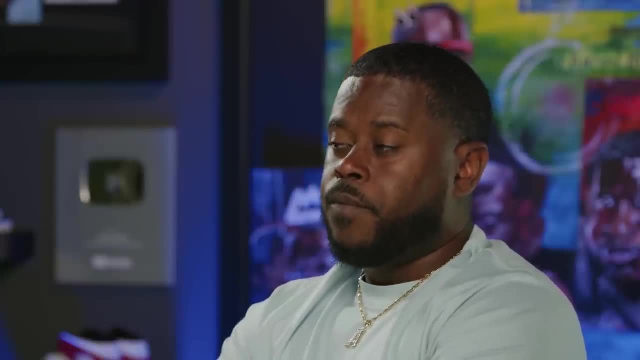 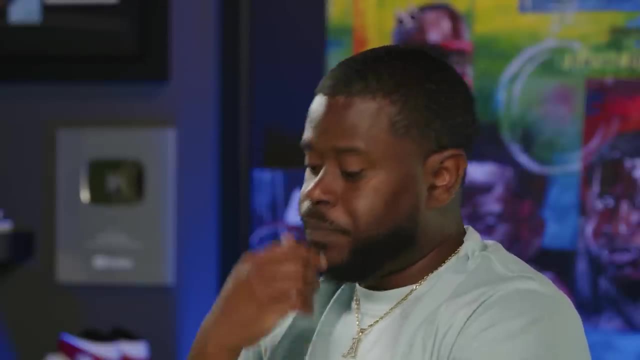 budget man. He said: I cannot find the money. I can't. I just I just can't get it. I don't know what's going on. So my RK cool. I said, Hey, what's what you're going to do? I said when you. 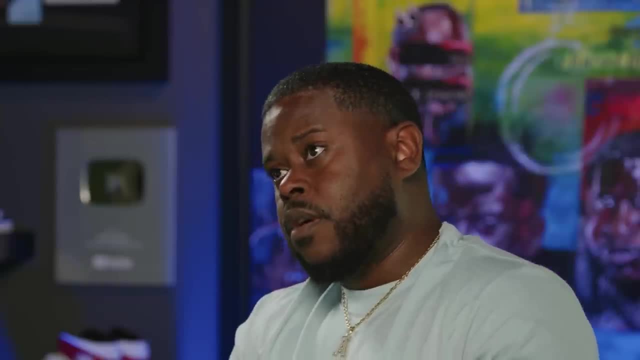 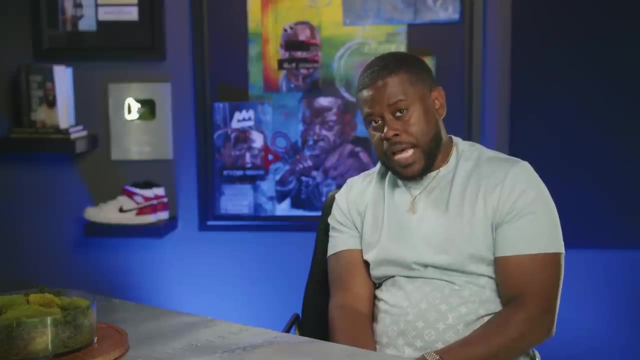 come, bring your last three months bank statements, bring your credit report, And when you sit down, we're going to go through it. We're going to sit down and see, okay, exactly where your money's going at. He was saying: man, I need to find at least another $300 in my income just to give me a little. 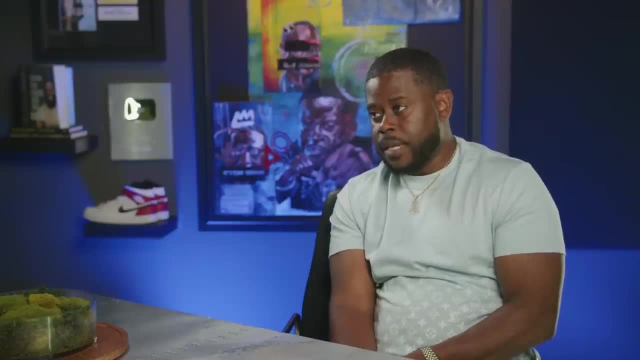 $300 breathing room. I said, all right, cool. As I'm going through his bank statements, I started seeing some um, I won't say that the particular name, but I started seeing some items on his credit- not his credit- on his bank statement- And I was like: what is this? What is this? What is? 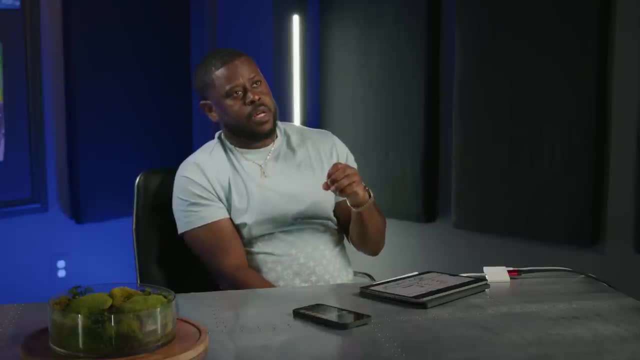 that. What is this? And I've seen it consistently, every um other day, every three days, I would see this charge, I would see this charge. I'm like: Hey bro, what's going on? I'm like I'm. 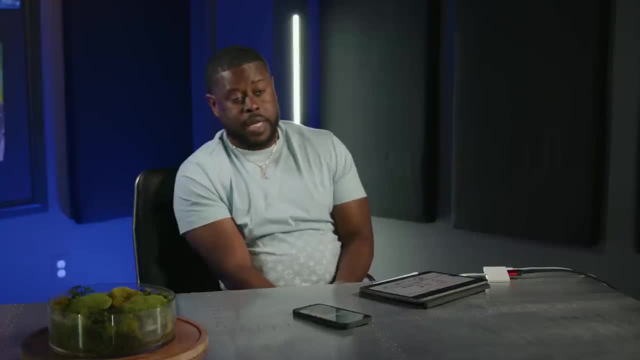 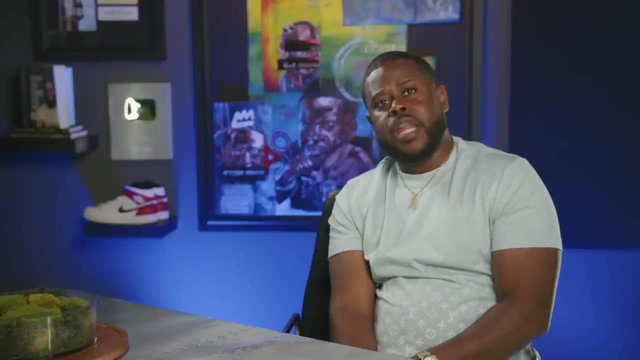 like: Hey bro, what is this? And- and I'm just being honest with you all, I'm not saying no names, where, where this particular brother is from, Cause I don't want to give away his location, Uh, but he had a porn addiction and he was buying certain things And I said: well, 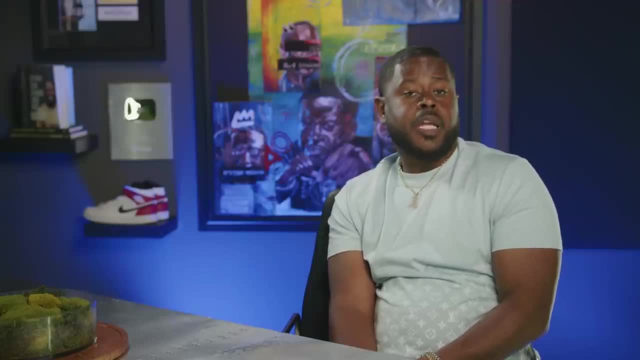 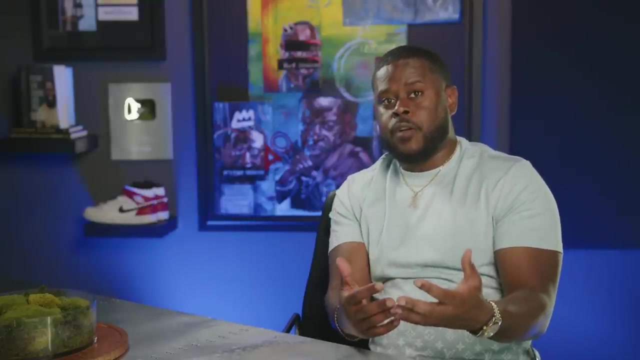 Hey bro, the problem here is not the money. The problem is you And I. I told him. I said: Hey, number one, surface level, you got to stop doing that. That's where your money's going. But if you really need this, if you're feeling as if you got to spend money like this, to please. 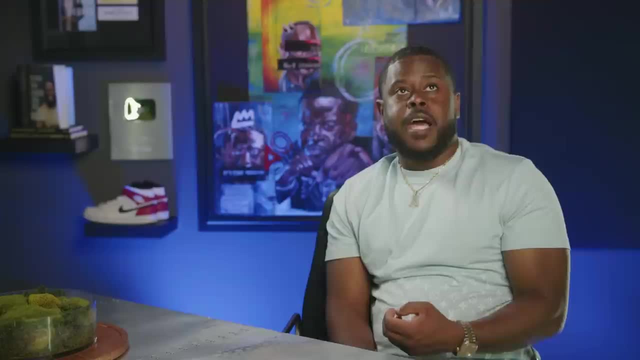 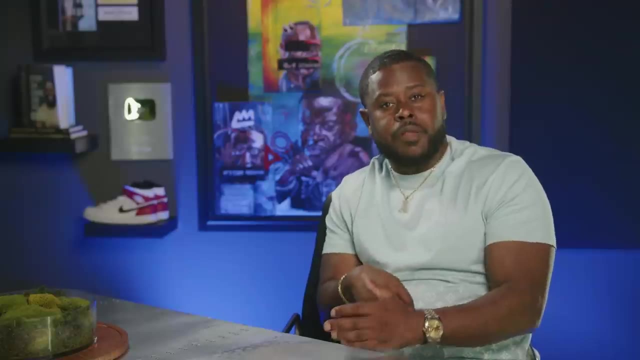 this need of yours. there's something deeper there that you need, that you need to go seek actual help for not saying that he's sick Cause he's not sick, but like there's something down that he really hasn't learned about himself and he's covering up by buying porn And I'm like so. 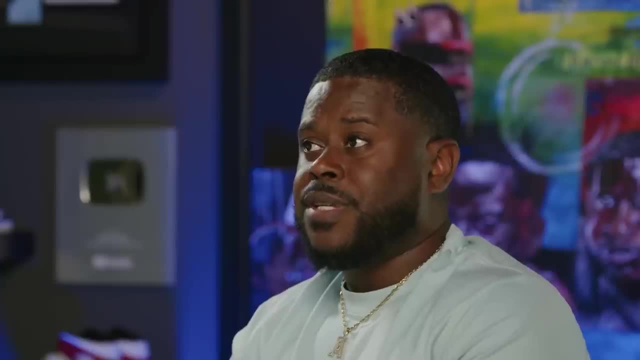 when it comes to adjusting your budget. you got sometimes. you got to be real and get around someone who will be very honest and transparent with you. I'm going to do it in a loving way. I would love to have you a part of this, because I believe that